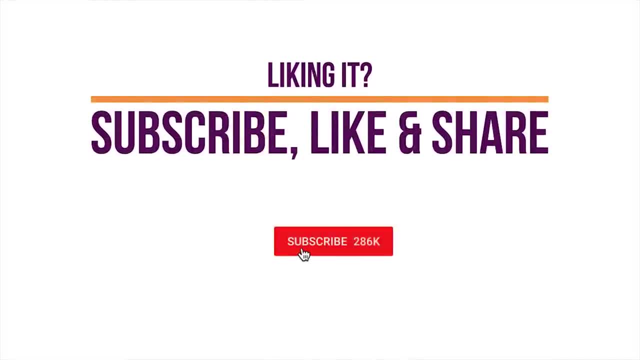 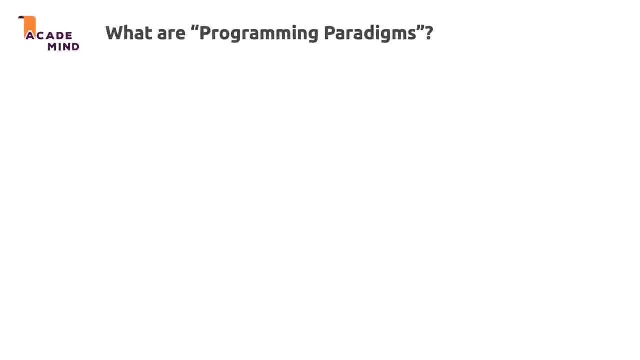 So what are programming paradigms? That's, of course, important to understand. In the end, you could say it's just a way of writing code. It's about how you write and organize your code. It's not a syntax feature, It's not a special feature exposed by the browser or anything like. 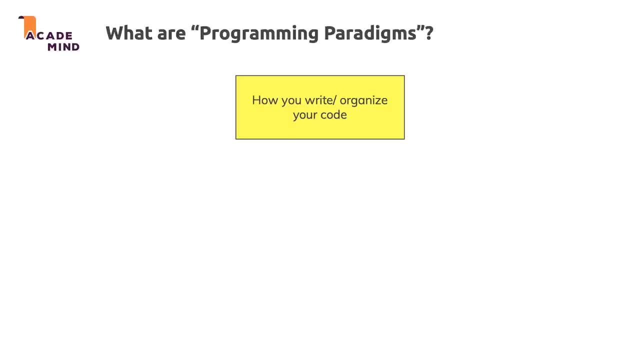 this. It's really just how you structure your code and how you reason about your program, your writing, so how your code is organized, And in the end there are three paradigms you could follow. You have object-oriented programming, you have procedural programming. 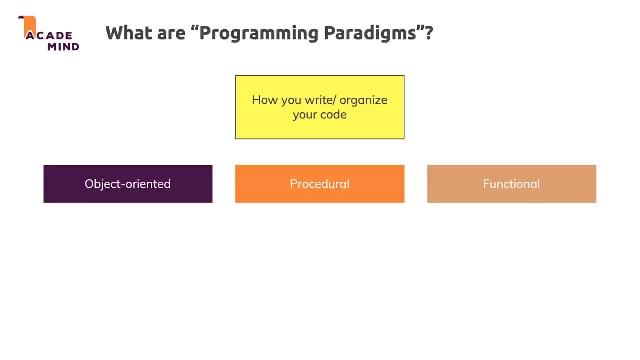 and you have functional programming. Now, what does this mean? If you're writing your code in an object-oriented style? it means that you organize your data and logic in objects or in classes, and then in objects based on those classes, which means you store your data. 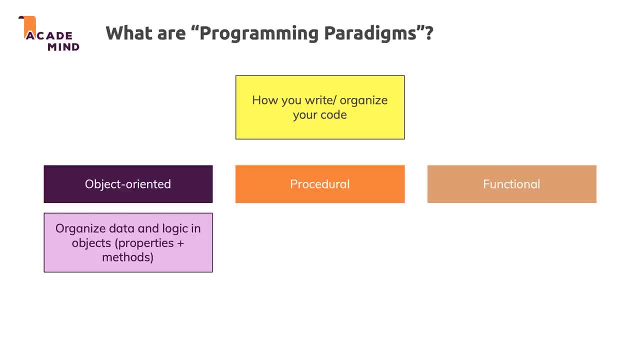 in properties of objects. You store your logic in methods of objects. That's how you typically think about your code. here Everything in your application, in your project gets represented as a class and then in the end as an object. So you organize your code in logical entities. you could say You kind of try to translate the 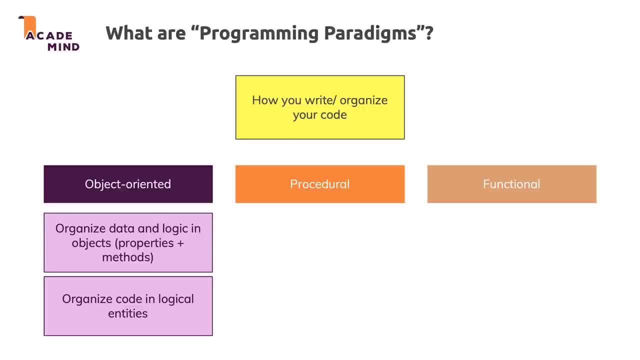 application, you're writing into the real world And you think about your application and the things that you're writing And you think about the things that you're writing And you think about the things that make up your application in real-world terms. If you're building a shop, 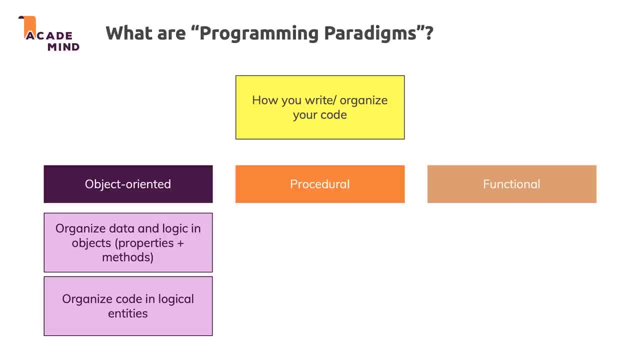 application. you think about products and a shopping cart and so on. That's how you think about your code and how you organize it Now, when you're following a procedural style, and that's probably the style with which you got started when working with JavaScript, 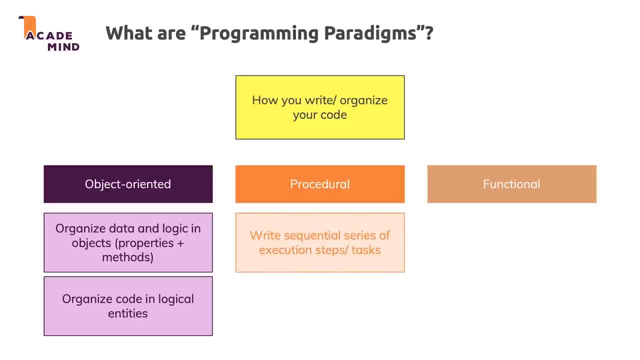 you simply write a sequential series of execution steps and tasks, So you have a top-to-bottom code execution. you could say: Now, you always have that in every style, But here you simply list these different steps. the engine in the end should execute and should perform. You don't organize. 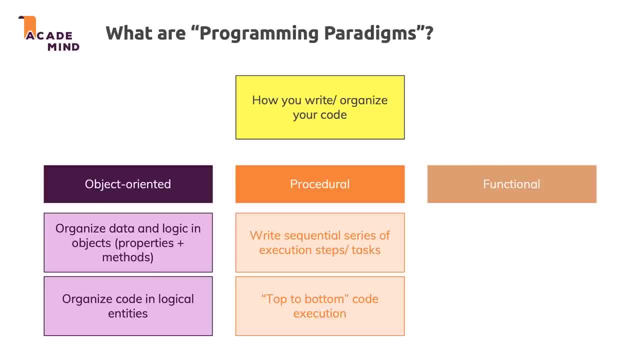 your code in logical groups or in logical pieces of data. You don't use objects and entities to structure your code. In the end you just execute step after step And then we have functional programming And there we organize our code in if possible. 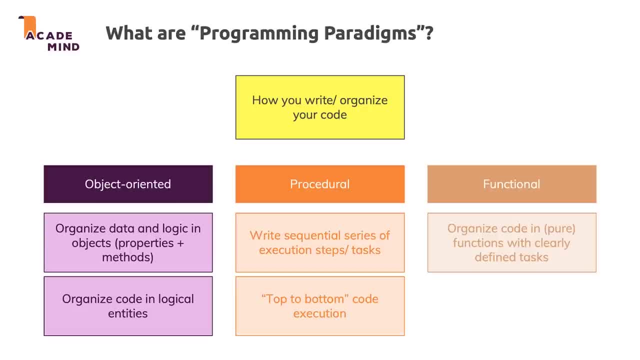 pure functions with clearly defined tasks. You get all the data a function needs as parameters, and then this function often also returns something new. So you pass data around with parameters and your functions are your way of organizing your code. You have many functions. 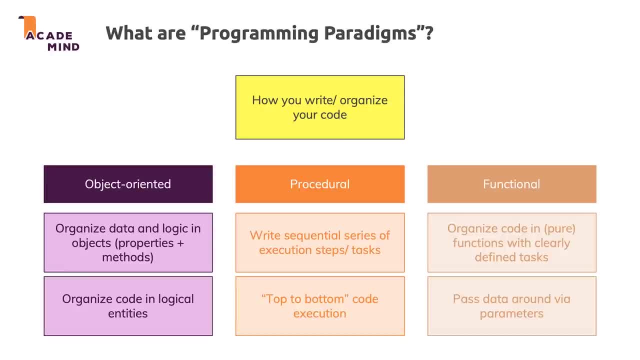 probably more than you have in the other styles, and your functions hold your logic. Every function, if possible, works on its own, And this is how you structure your code. Now, that's the theory. It, of course, becomes way clearer if we see that on a real example. 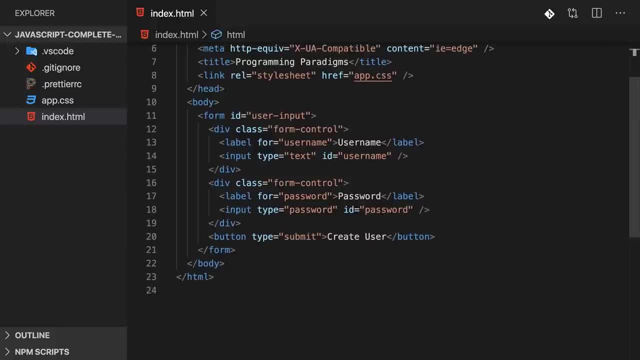 So let's work on a very simple example application, And this, indeed, will be a very trivial application here. It's an application where I, in the end, have an HTML file which renders a form- a form with two inputs and then with a button, And I got some styling so that this 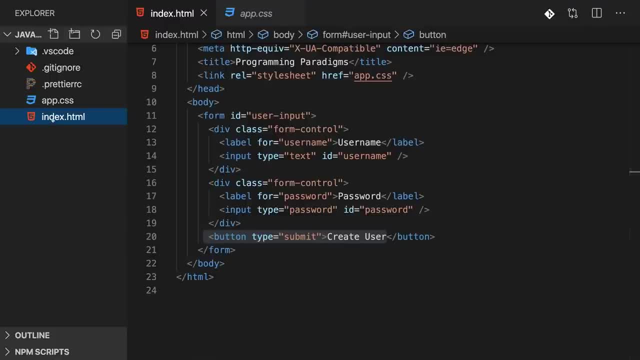 doesn't look super ugly. Now we can simply open this by, in the end, double-clicking that index HTML file in the file, And then we have a very simple example application And this, indeed, will be a very simple example application, And this, indeed, will be a very simple example application. 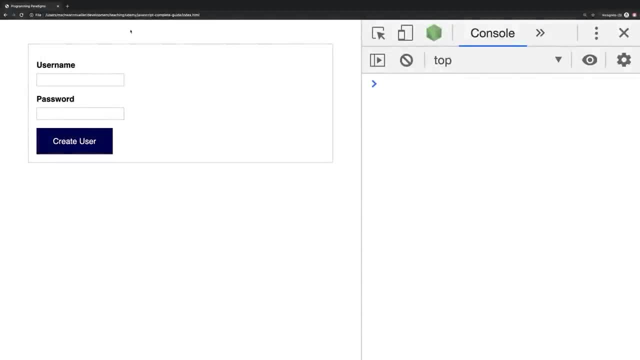 And this, indeed, will be a very simple example application, And what we get is something that looks like this: Now here, nothing happens. If you enter something here and click the button, you'll just submit the form and therefore reload the page. Besides that, nothing will happen. 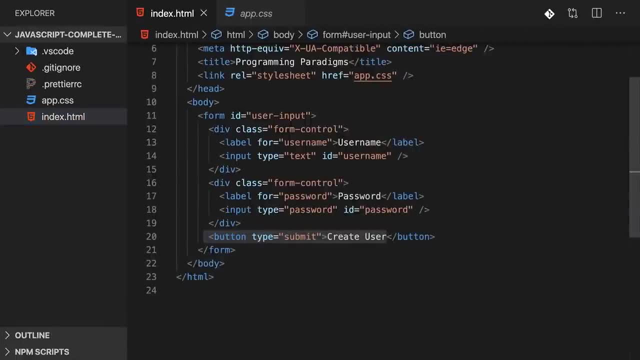 We will now write code that changes this And we will write this application code three times in the three different programming styles. And we'll start with procedural because, as I mentioned, this might be the style you use for your code. And we'll start with procedural because, as I mentioned, 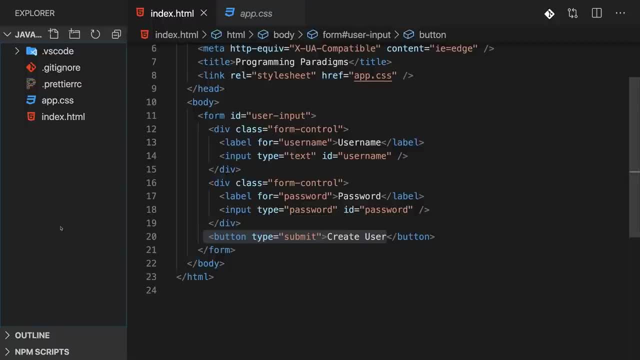 when you started with JavaScript, because I would argue it is the style that's the most obvious to use if you're getting started with programming. So let's add a new script here, proceduraljavascript. You can, of course, name it however you want And in the index HTML file below that link here: 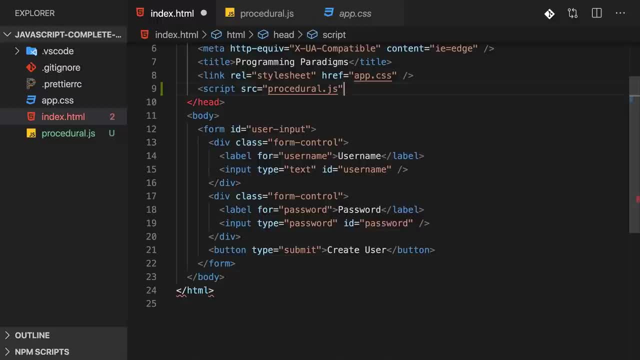 I'll add a script, import and point at proceduraljavascript, add the defer attribute to make sure that this script only runs after the entire file has been parsed And, of course, close the script tag as well. and now we are importing this and we're ready to write some code. 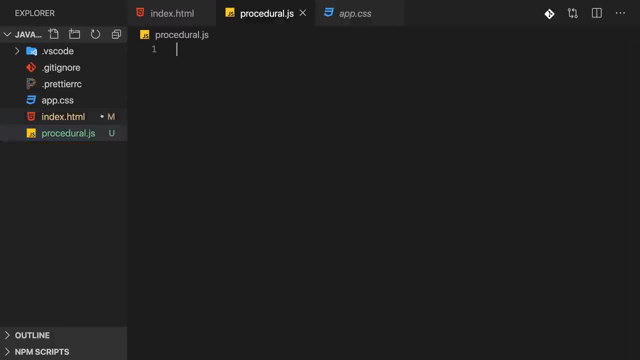 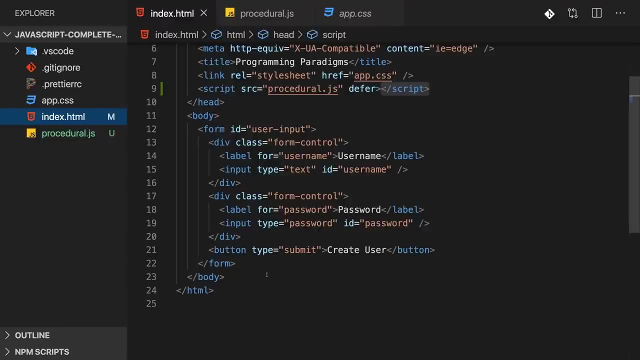 and now we can really think about the different steps we want to execute, because that's what procedural programming is all about. so, if we have a look at our html file, what do we want to do? well, we want to listen to a click on this button, of course. or, to be precise, we want to listen for 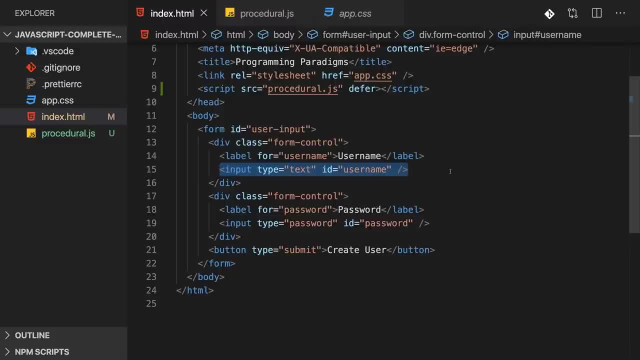 the submission of the form. we want to get the values to user entered for the username and for the password, and we might want to validate those values. so at least make sure both fields are not empty, show an error message if they are empty and then in the end, if everything has been valid. 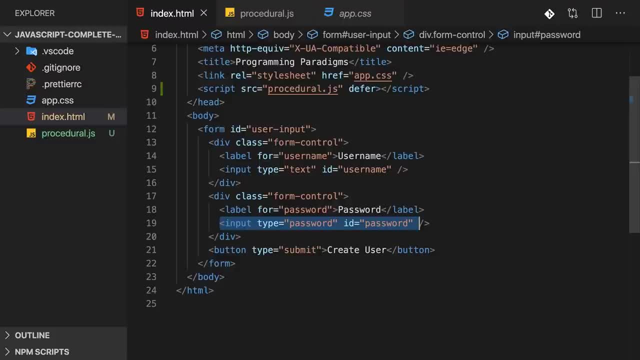 do something with the data, let's say, create a new object, a new user object, and then log that to the console or something like this. so something fairly trivial. that is what we could do here. so for that, back to the procedural js file, what do we do? 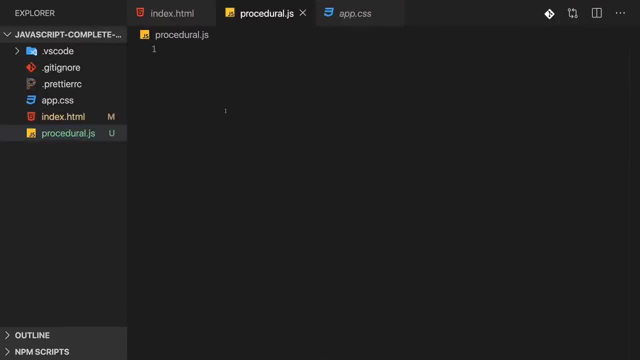 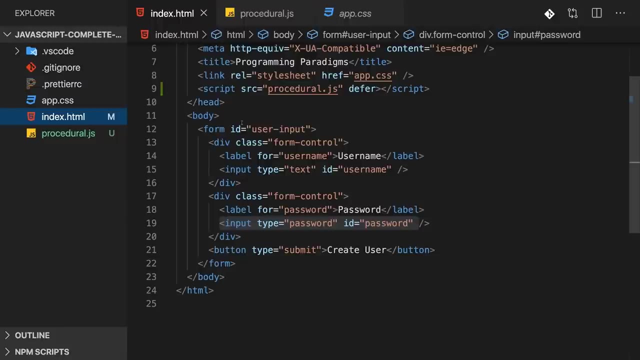 need to do here? well, we need to get access to the form and to the two inputs so that we can work with the data there, and then we can add a listener to the form and so on. so getting access to those things is easy. we have ids with the user input id on the form, with the username id on this input. 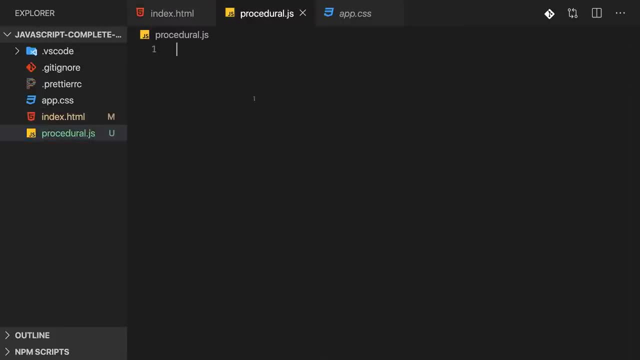 and the password id on this input so we can use these three inputs to gain access. so i'll store the form in a form constant, or i'll store a reference to the form in the form constant and we can get access with get lsd. and then here it was, user dash input and then the second constant i want to create here is the. 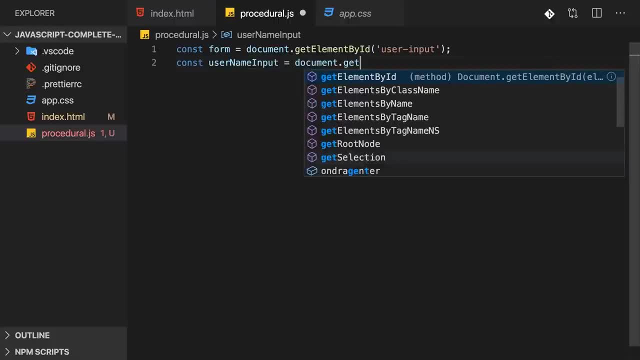 username input, we can get access with document. get element by id username and, last but not least, the password. so the password input that can be fetched with document, get element by id password like this. okay, so we get this access. let's now add an event listener. so on the form, 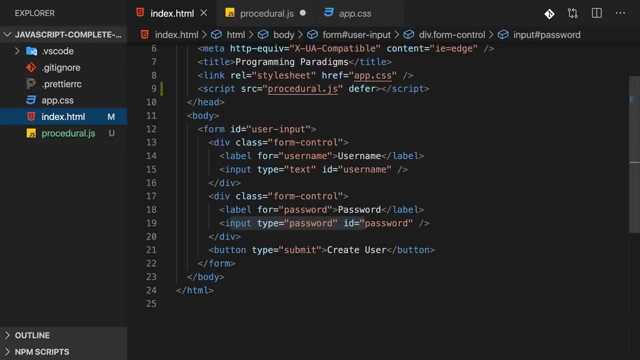 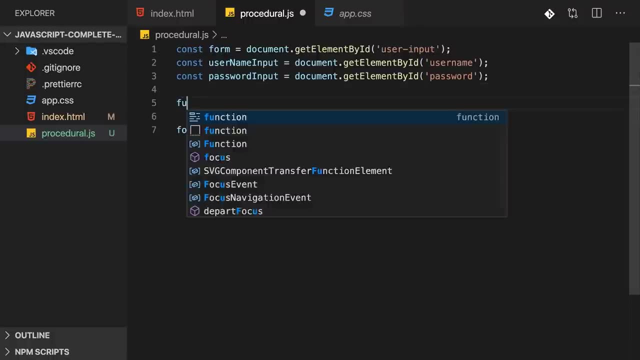 i'll add an event listener to the submit event, because that is the event we want to listen to, right. and then we want to trigger a function when that executes. we could use an anonymous function here, but i will create a named function, the sign up handler, let's say it will get an event object. 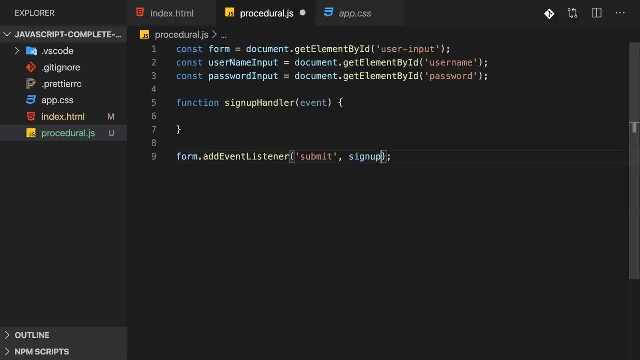 automatically- and i will point at this function- when this event is triggered, when this event is fired. now, this is vanilla javascript and, of course, even though we're using the procedural style, we are allowed to work with the event listener, so we can get access to the form and then we can. 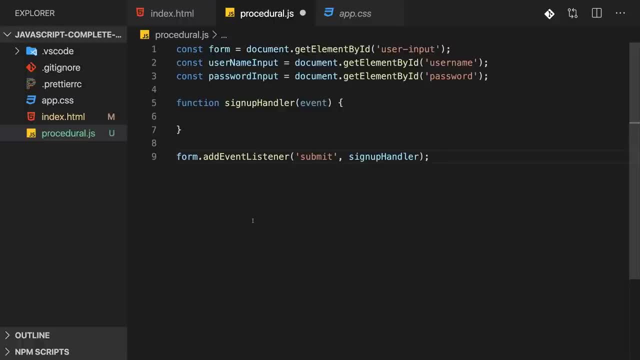 work with functions as well. this is not forbidden. we just don't organize our code around the idea of using functions all the time. so we point at this function here when this event is triggered. and now in this function we write all the logic again, step by step, which we want to execute. so 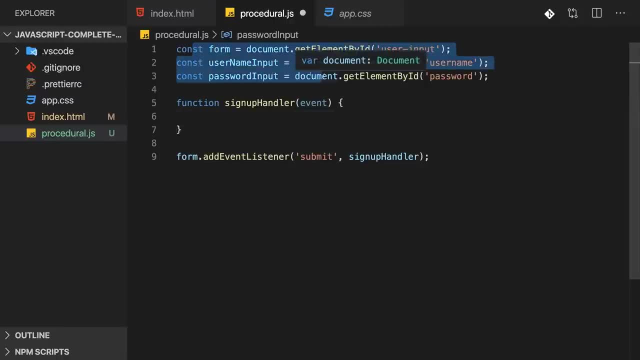 thus far, our logic is: get access to the different elements step by step and then define this function and then set up this listener. now, when this function runs, we need to get the input function, and then we need to get the input function, and then we need to get the input function. 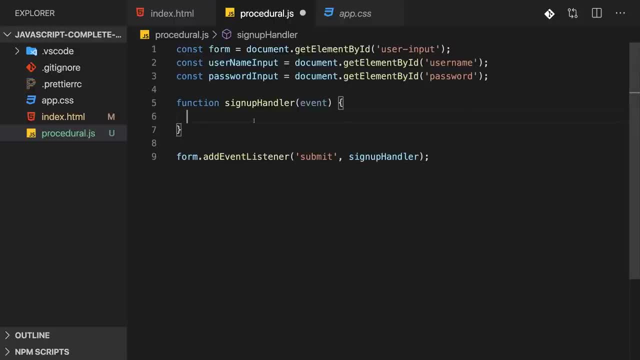 here the values the user entered. we need to validate them and then create a dummy user object with that data. and actually, first of all, i want to call event prevent default to prevent that browser default of sending the form to a back-end server which in the end leads to a page refresh which i 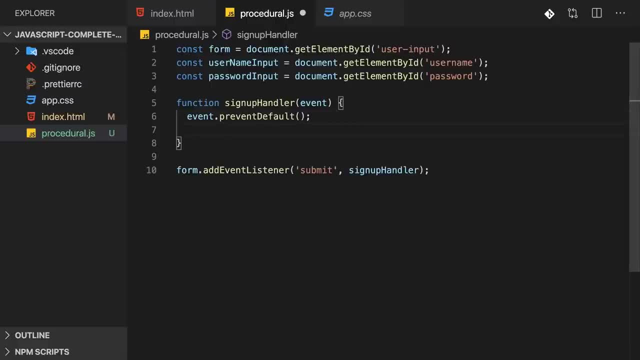 don't want here. so let's call this as well. and now we can get started. let's get the concrete values the user entered. so we got the entered username and we can get this out here and we can get the code of username input, dot value. we can access dot value here because we know that the element 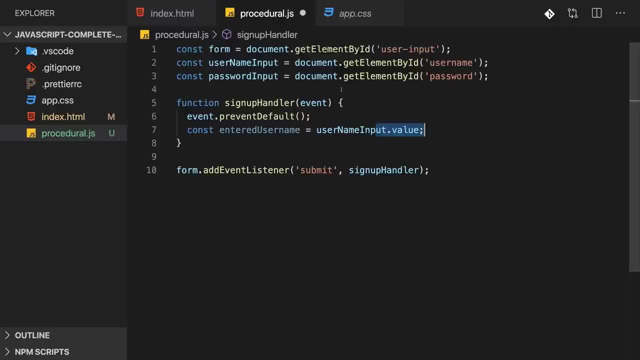 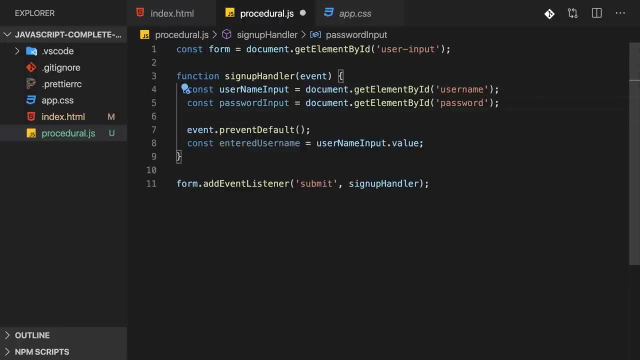 we're selecting here is an input element which will have a value property. side note, you could actually also only get access to the username input in here if you wanted to, because we really only need the two inputs here inside of this function, so you don't have to do it globally. 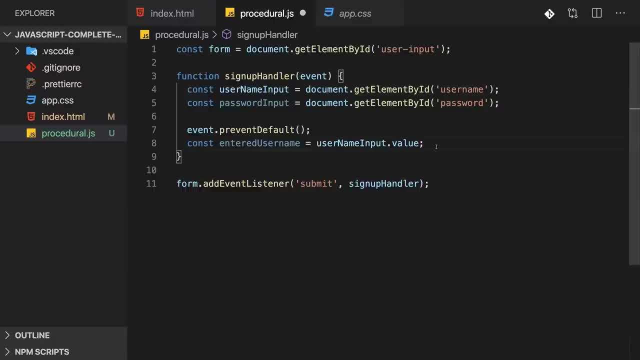 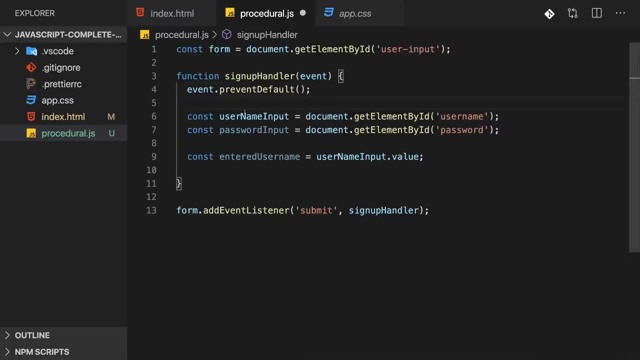 here in this function it would also suffice. so maybe let's reorganize our code to do that inside of this function. we have to do that in the default command and it's going to do that in the default command. we're going to get the value. that's not required, but it is a possibility, so we get the entered. 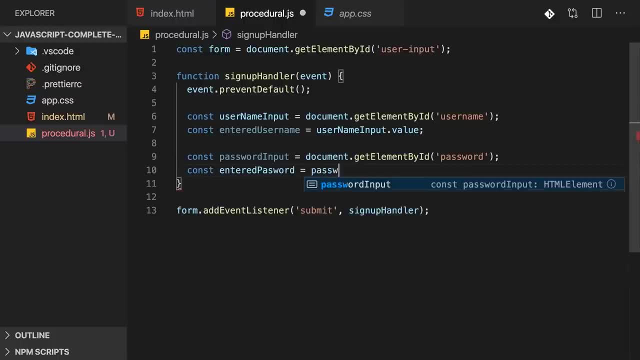 username, we can also get the entered password and we get that from the password input dot value, of course, just like this. now, with the two values, we can validate them. we could do this with a if check, where we check if the entered username, if we trim it to remove x's white space at the beginning and 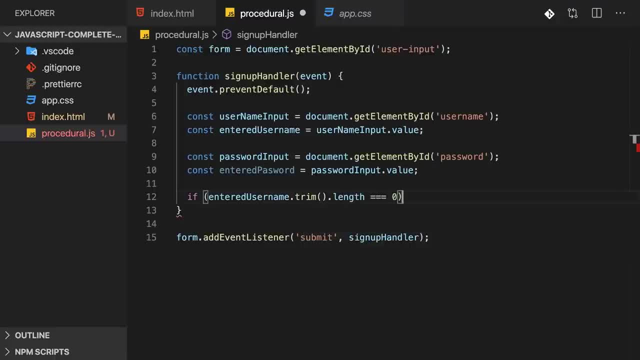 end if the length is equal to zero, which means This is an invalid input. it's empty. In this case we could show an alert to the user and say: invalid input. username must not be empty. That's something we could do here, and we also return here, which means we cancel this function execution so that we don't continue in the code. 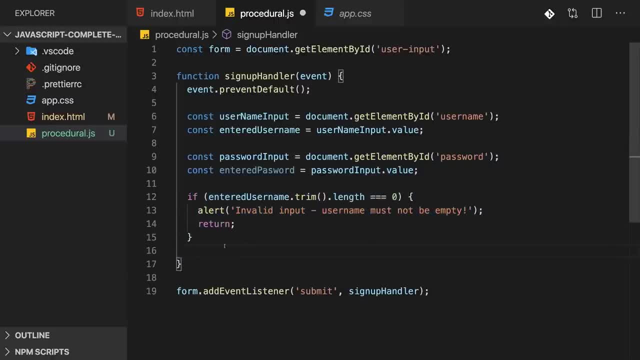 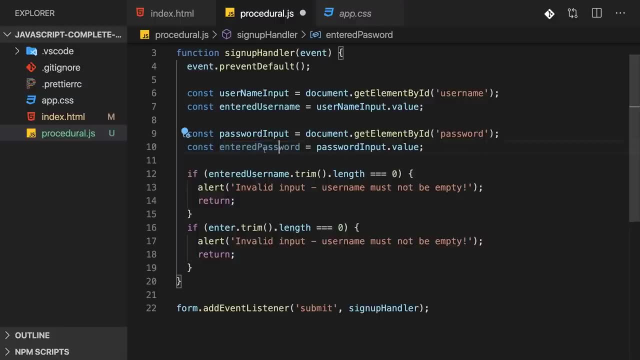 If we make it past this, if check we might still have an invalid input because our password, our entered password, whoops with a double S here entered password. that might also be wrong. So we trim this and check if the length is 0 or maybe if it's smaller or equal than 5, because let's say we want a password which has at least 5 characters. 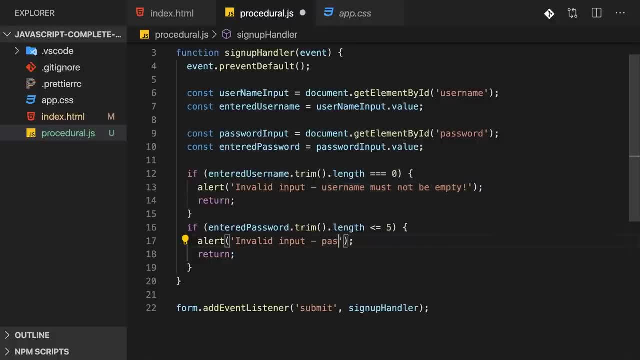 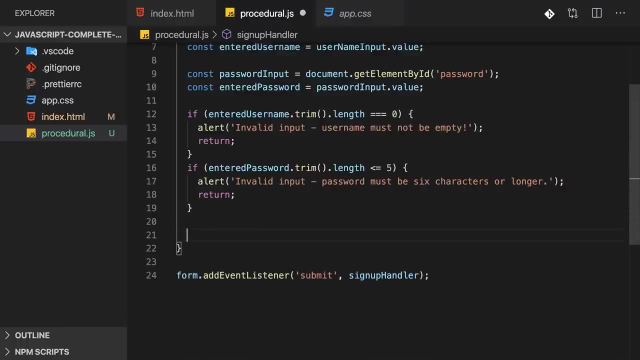 If it is too short, we can say invalid input. password must be 6 characters And again, we thereafter return so that we don't continue with the function execution. If we do continue, we made it past both if checks and we now know we have a valid input. 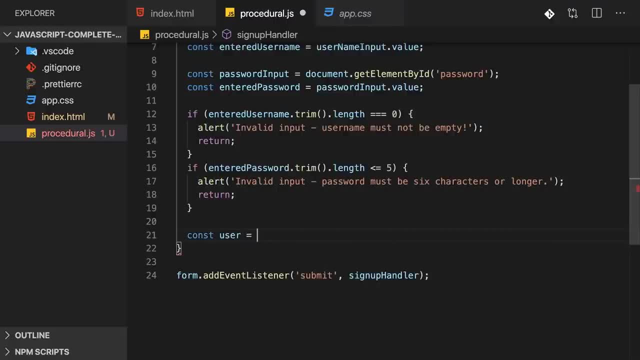 And that's where we now could create a new user object simply with an object literal. Again, just like functions are not forbidden here, objects are not forbidden here. It's not like you're only allowed to use objects when you're writing object-oriented code. 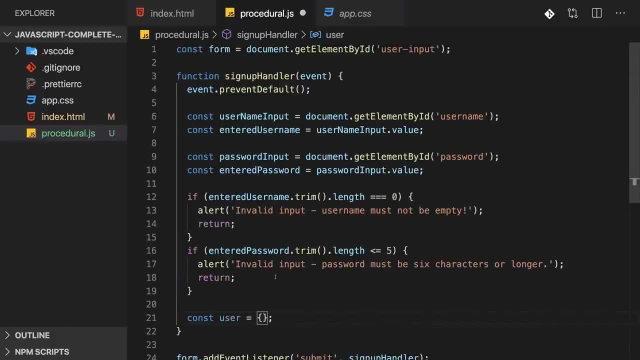 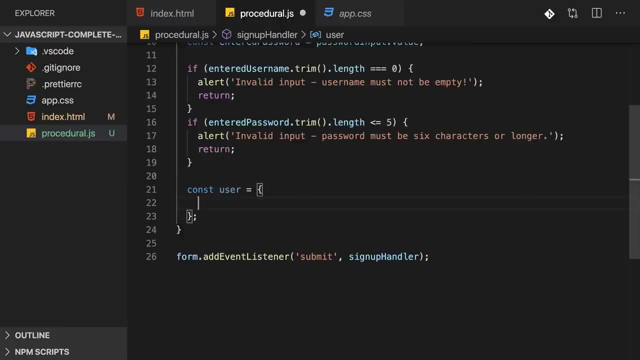 It's more about how you organize. It's more about how you organize- And here it's really a step-by-step execution, and we're using a very simple literal object here to store some data, to group some data. So here we then have, let's say, the username, which is our entered username. 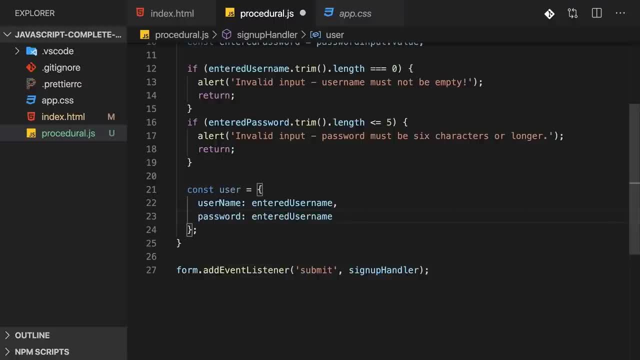 We have the password which is our entered password, whoops, entered password And with that we're good, And now we can console log the user and maybe also send a greeting with hi, I am plus useruser Name like this: 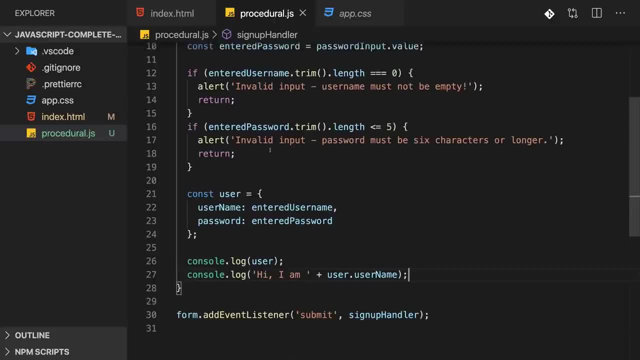 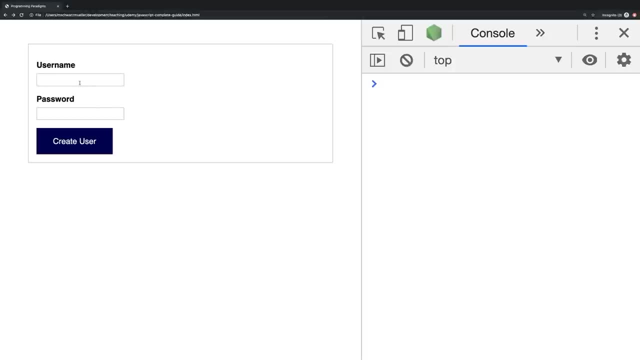 With that we had a very basic procedural program. If we now save this and we go back to the browser and reload this page, if I enter Maximilian here and then any password of my choice, which is, let's say, too short actually, I get this error. 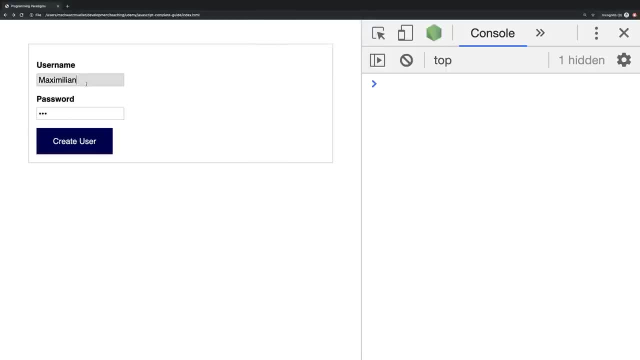 Invalid input. password must be six characters or longer. If I don't enter Maximilian here but I leave this empty, I get this error regarding my username. and if I do have valid inputs in both fields here, you see, we're logging the user, we're logging hi. I am Maximilian. now, as I mentioned, this code here should look fairly. 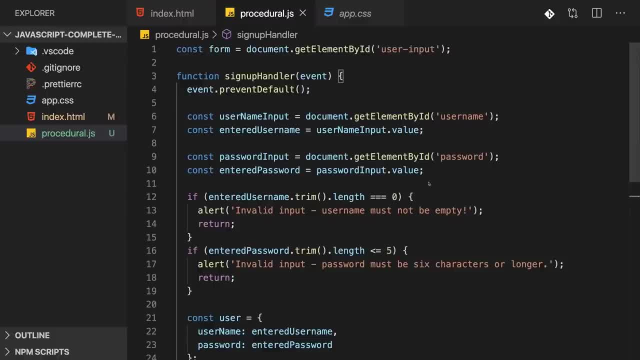 straightforward to you. there also is nothing wrong with it, but this would be the the simple, procedural way of writing your code. you think about the different steps you need to execute and you then just write them down. and don't get me wrong: code will always be executed from top. 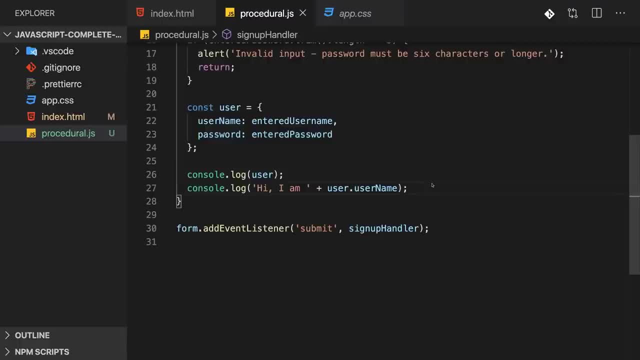 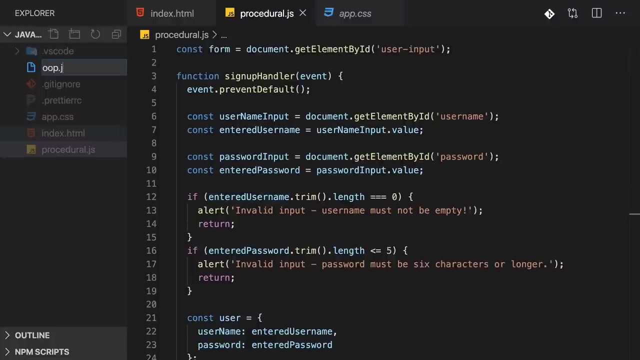 to bottom. but you could also organize this differently. so let's have a look at the object oriented programming style next. so we wrote this code here in the procedural style. you could say: now let's create a new javascript file, oopjs, where we will write basically the same logic. 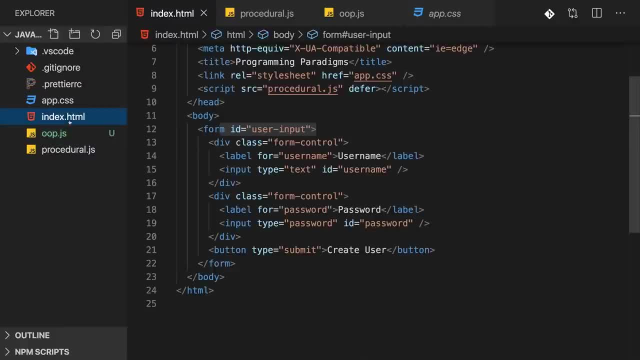 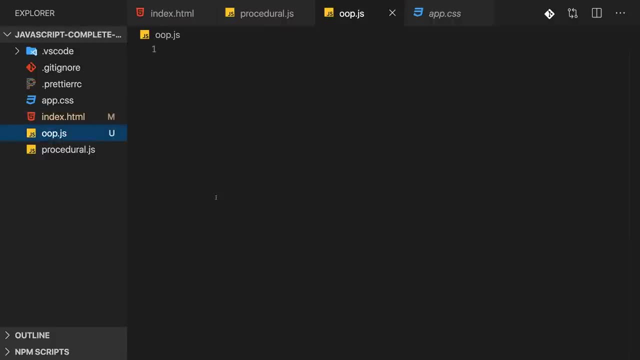 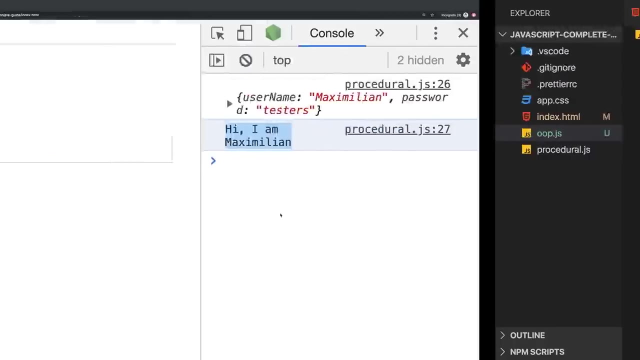 but now using an object oriented. style you so for that in indexhtml, I'll swap the import for the oopjs file here. now, how would this look like if we think about this in an object oriented way? now, there are certainly different ways of approaching this, but I would like to think about the different entities, the different types of 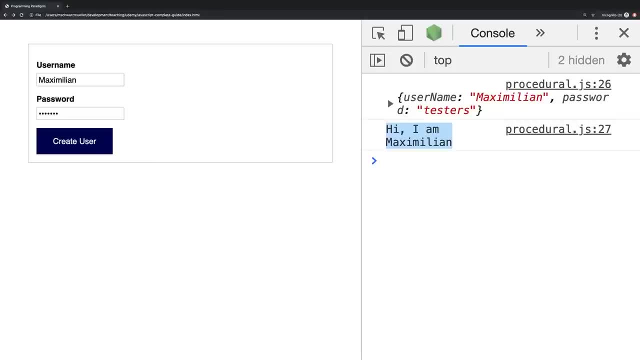 objects we could work with here. we could say our form, for example, is one object. it's one object which in the end will have two inputs, which has this button and which will have a method which is triggered when the button is fired. the validation could be organized in its own object. 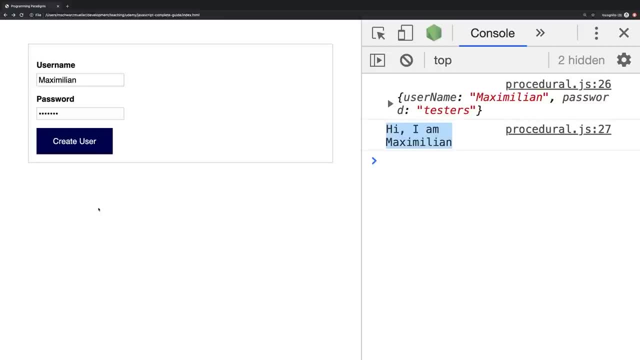 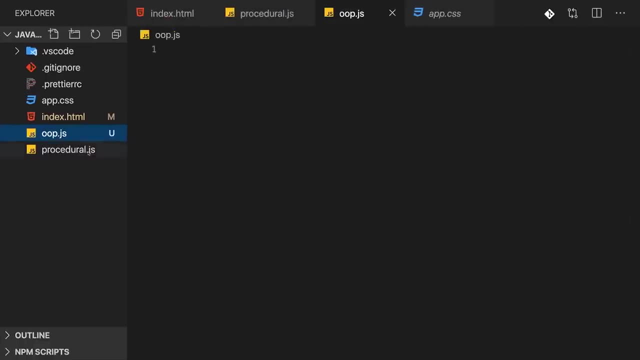 as well in a helper object which holds validation logic that we could reuse in different parts of the application. if we had multiple forms and the user we create in the end, well, we could create a blueprint for this user as well, a class or a constructor function which allows us to create. 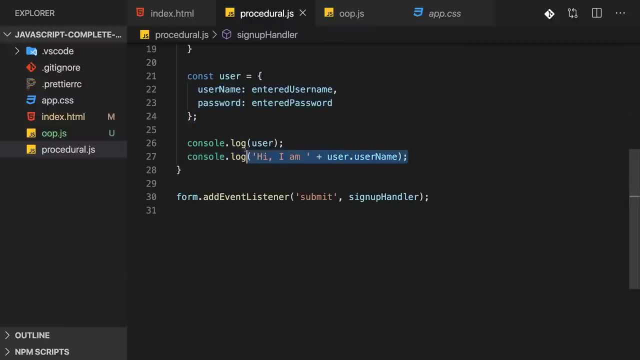 user objects which has a built-in greet method to show this greeting, for example. so here we have a function with the same name and we can write a class text which, as we can see it, can be used in multiple ways, but instead of just setting it up here in the object or in hit javascript file, I 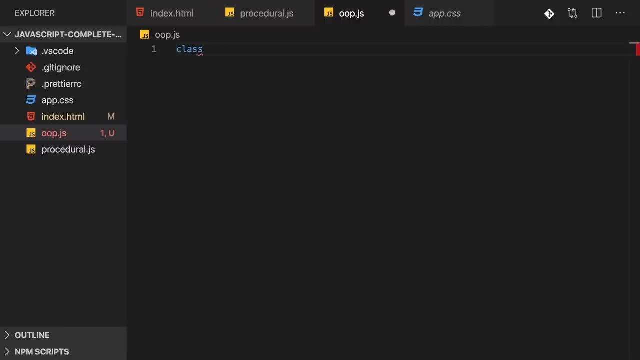 will work with classes. if you were working with an older version of javascript, you could of course also work with constructor functions instead. classes in the end, are just syntactic sugar with some extras, and you learn all about that, of course, in my complete guide, in the object oriented and. 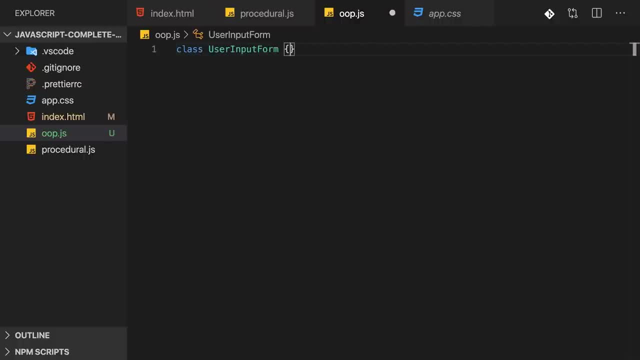 classes, core section. so which classes do we need here? well, we have our form right, so I'll add a is related to my form. i also want to have another class, and the order does not really matter here. i'll just have the form at the bottom, because it is the thing i will actually, uh, start with, and it 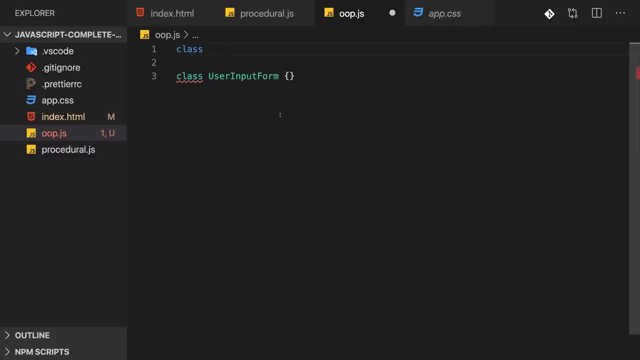 will use all the other classes which i'm about to define, so i want to define them first, though technically, as i said, you could also organize this differently. but here, another class we'll need later is the user itself, so not the input form, but for the concrete user object we work with. 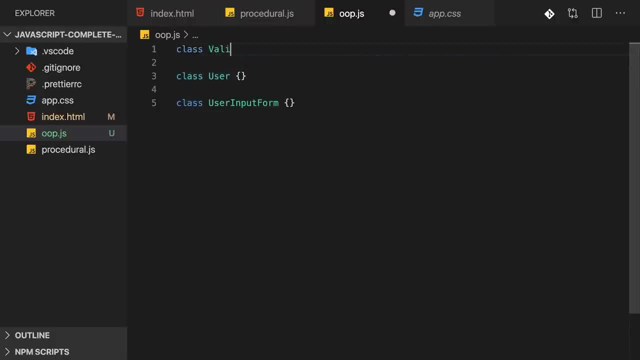 and then maybe also our validator class here, which holds our validation logic. now let's start with the user input form, though. what could be in there? well, i want to define my constructor function, which allows us to do some initialization work whenever we create instance based on this class. now, my goal is to create an instance based on 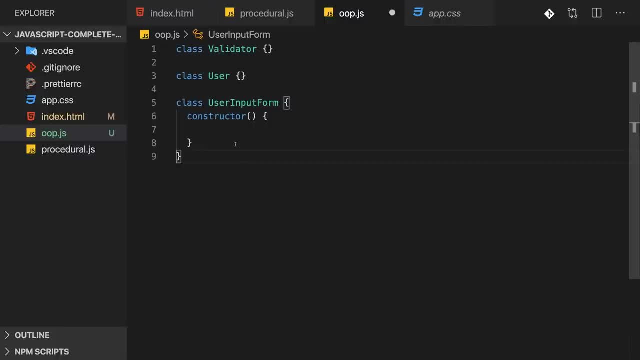 this class when the app starts in the end. so therefore, here i want to get access to the different inputs- inputs in the HTML file- and to the form itself, so that we can add a listener. So here I will add some properties to the instance created based on the class with this keyword, For example, a form. 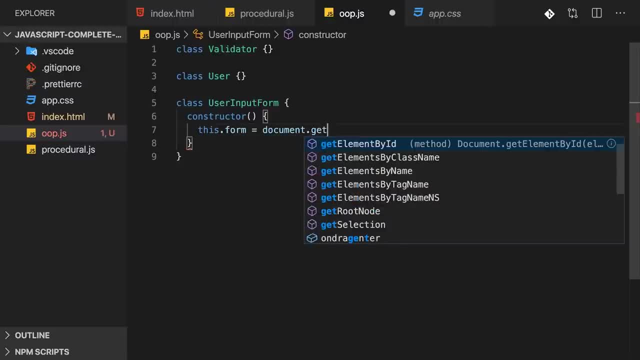 property and the name is up to you. And here I get access to get element by ID user dash input. So here I store access to this user input form. I also want to get access to the different input fields in the form. So I have my user name input field document: get element by ID user name And. 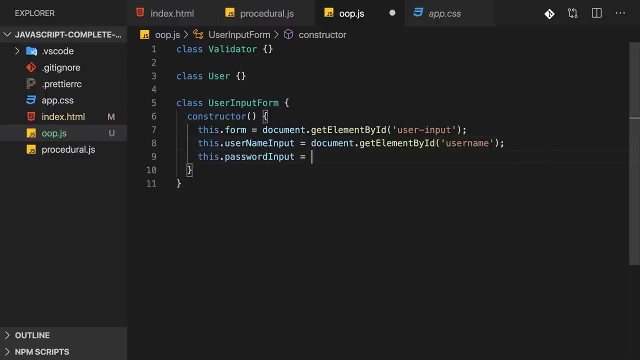 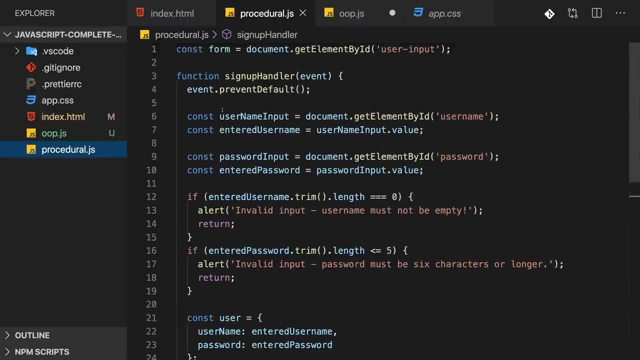 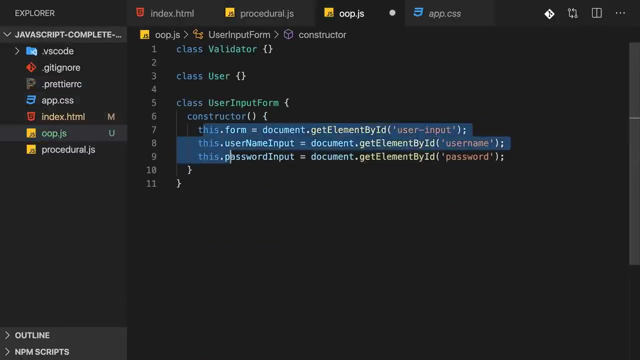 of course, one for the password. So password input with document, get element by ID password. So basically, what we stored in constants before here, this constant, this constant and this constant is now getting stored in properties of this class. or to be precise, 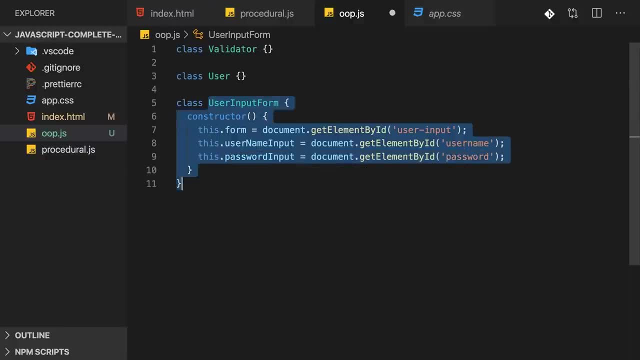 in properties of the concrete objects created based on this class. I also, of course, will reach out to my form and add an event listener here for the submit event And when this is triggered. of course, once you trigger a function Now, we could work with an anonymous function here. But 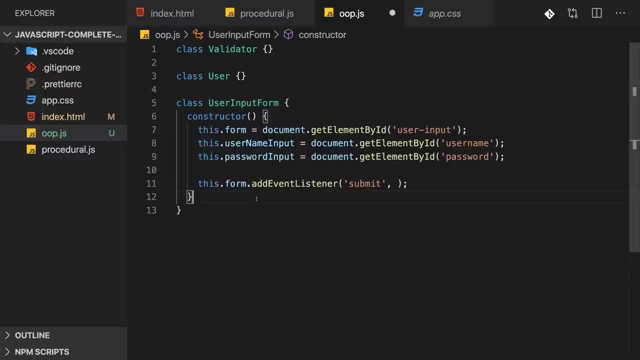 since we're in a class and we want to write object oriented code, it makes much more sense to create a method, So a function inside of an object, inside of a class, here. So for that I'll add the signupHandler method here. 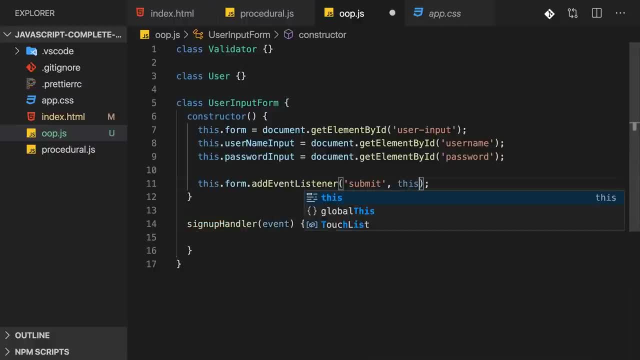 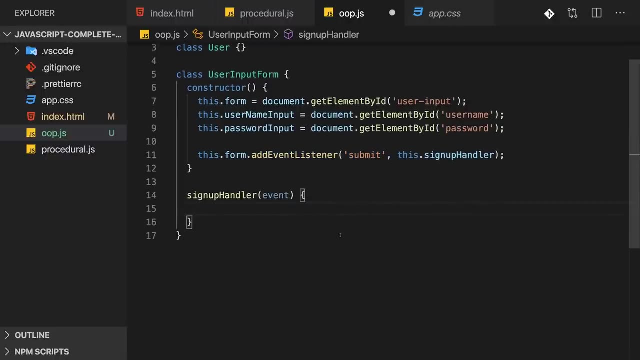 which gets the event object, And now I can point at it here- this signupHandler. This ensures that this function, which is registered on this class and which therefore is called a method, is fired whenever this submit event occurs. And in here we can now do stuff. 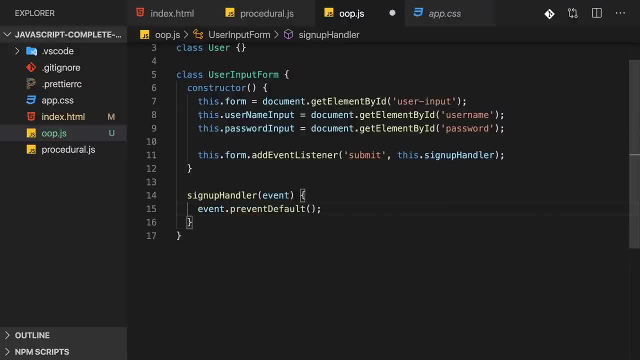 We can call event prevent, default, but we can now also get the concrete entered values and validate them and so on. Now one important word: if I want to get the, let's say, entered username here, then I of course can reach out to this username input. 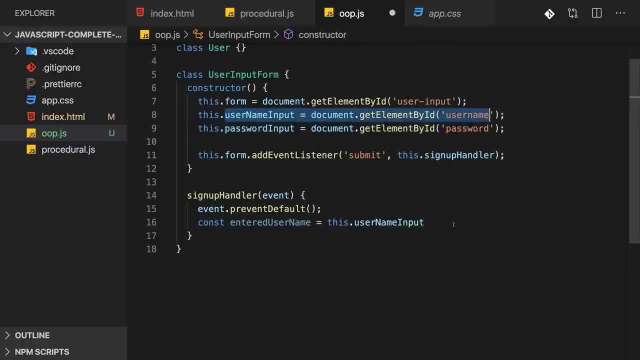 so to this pointer, at this input element in the HTML code we stored here and accessvalue, But this won't work. Why won't it work? Because this keyword inside of this method will not refer to this class, in this case here. Why? 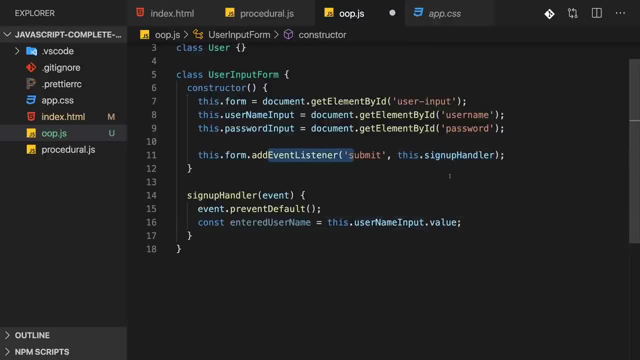 Because this method gets fired upon this event And when you point at a function or a method based on an event, that gets triggered. so here, on such an event listener, the, this keyword will be bound to the event target. That's a default behavior. 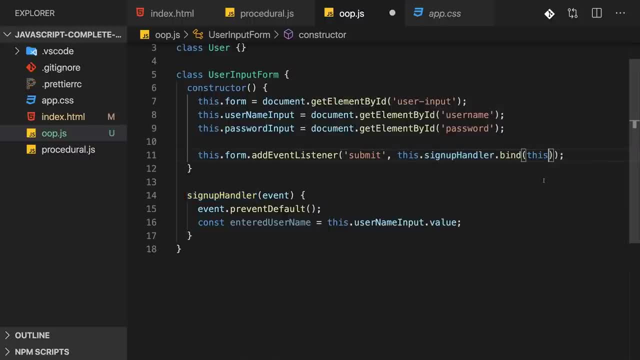 To override this, we have to call bind this here. This ensures that the this keyword inside of signupHandler will point to the exact same thing this would point to in the constructor, And that will be the instance created based on the class. So now this will work. 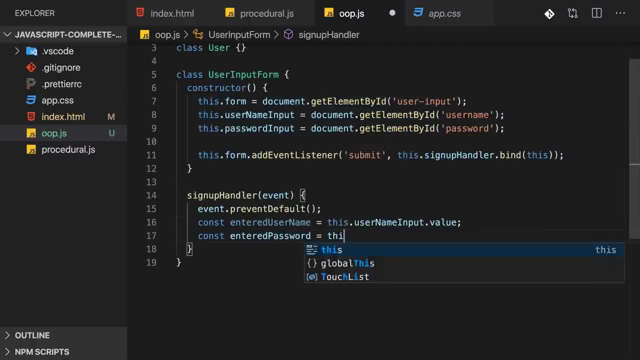 Now let's consider this empty inner line here. This is exactly what we could use to add value to our wrapper Als. Let's call it Password, which is that we can pickup from the bite dot value, which is actually the values that were used to add value. 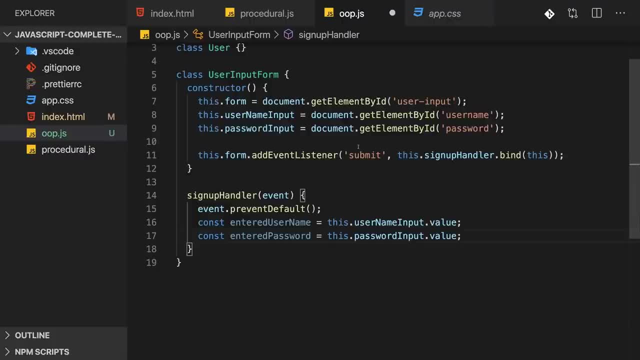 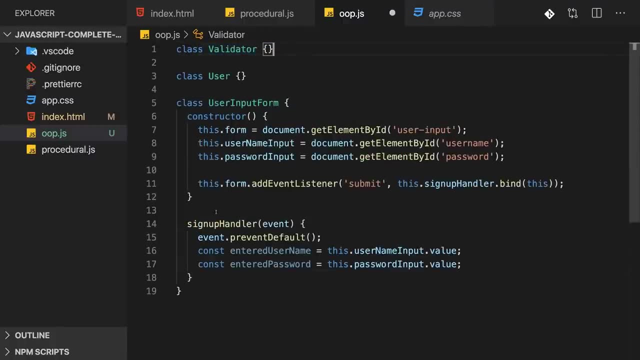 to that current wrapper, aluminum. If we do this correctly, we can therefore also get the entered password here with this password input dot value. So now we get the two values, now it would make sense to validate them And here again thinking in an object oriented way. 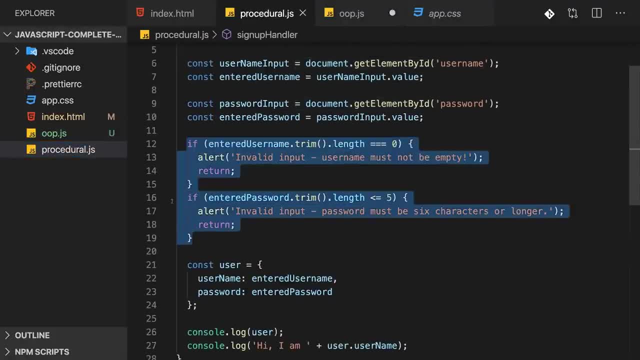 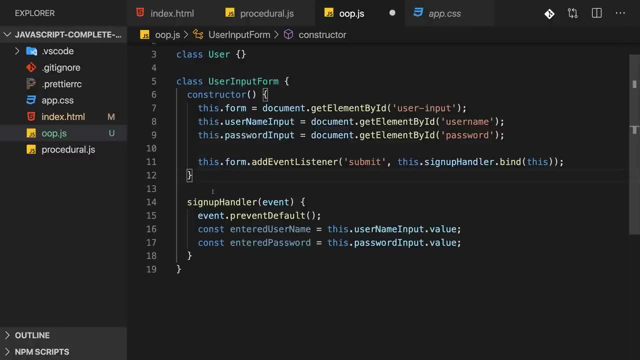 we could outsource this validation logic into a validator class. We don't have to do that. We could write it inline here. We could just copy over. we can only reuse our code by copying it again. And copy and pasting is not something you want to do too often. 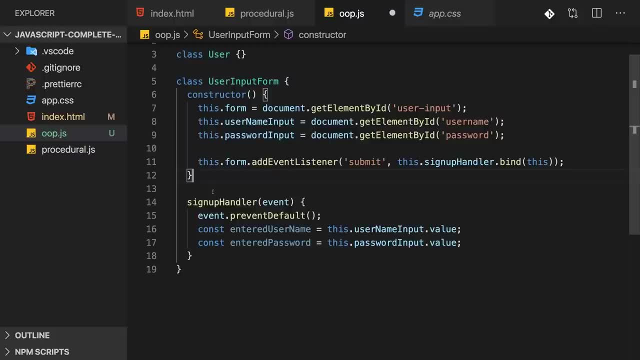 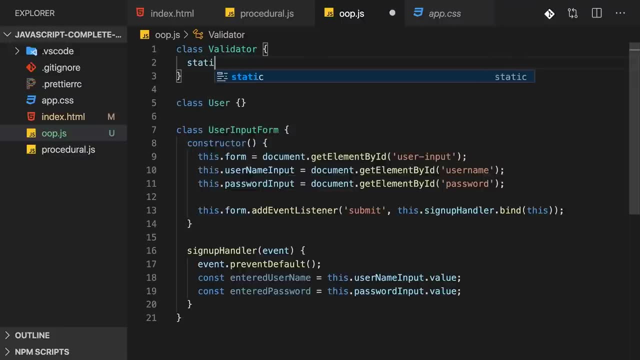 because that is a bad programming style. You're repeating yourself and you shouldn't do that. So instead I'll add something here. in the validator class, I'll add a static method: validate. This means we can call it without instantiating this class. 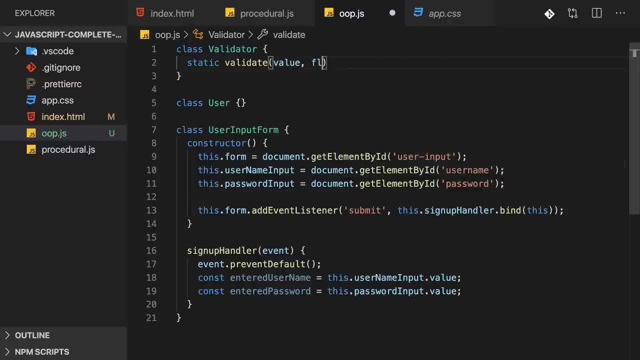 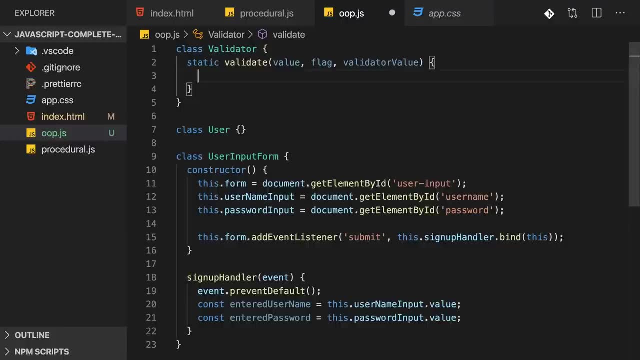 And there I expect to get a value. and then let's say, a flag and a validator value, if you want to. So I'm writing a little bit of a more complex validator here. What does this mean? Well, value should be the value I want to check. 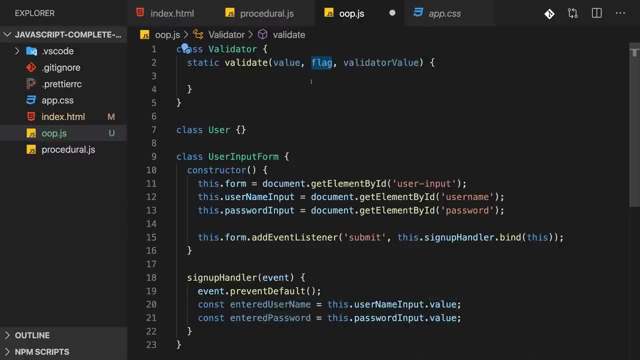 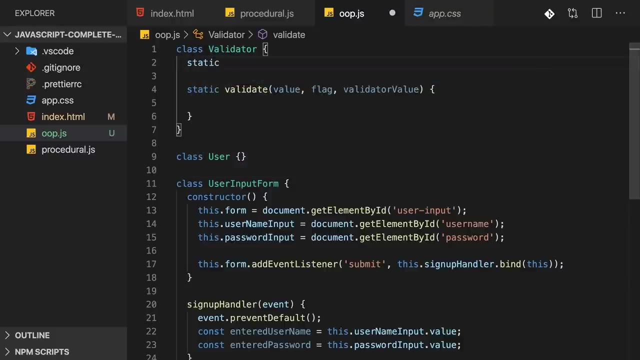 So the entered username and entered password Flag should then allow us to identify which kind of validation we want to perform, And then validator value is basically optional, allowing us to configure the validation. Now, for this to work, I'll add two new static properties here. 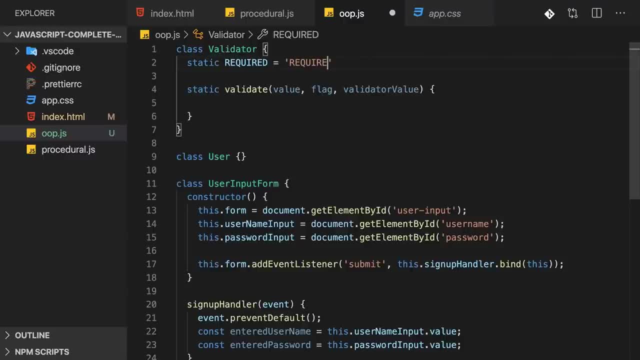 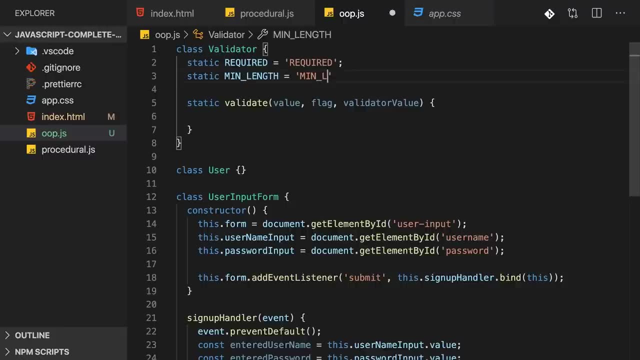 Required, and I'm writing it all caps to make it clear that this is the value I want to check. This is basically a globally unique value, you could say, And min length here, And these are just identifiers which we can then use. 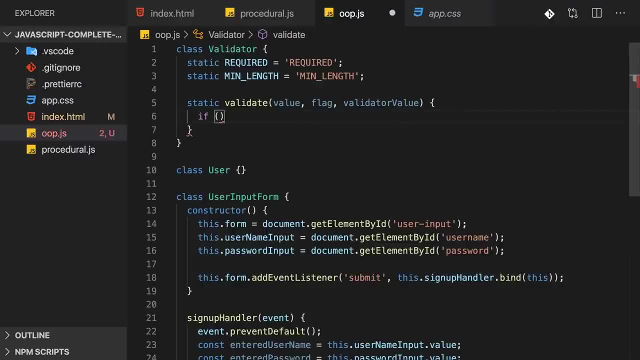 Because my idea now is that I can check if in here in the validate function, if the flag argument I'm getting, if this is equal to this required, So if we're running some required validation. And if it is, I want to return true or false. 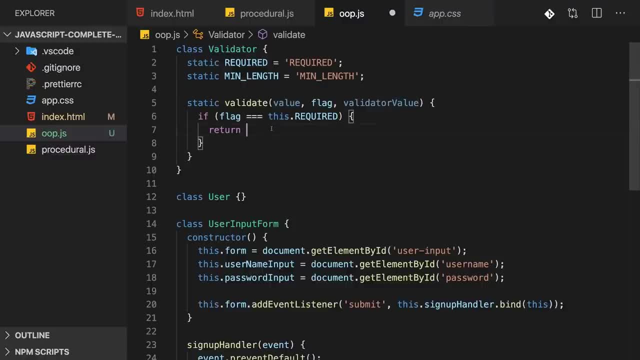 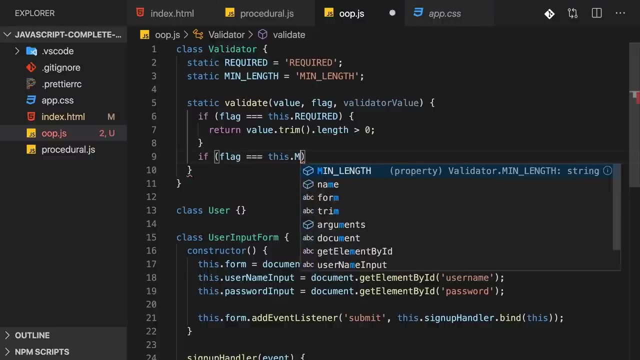 I want to return true if the entered value is not empty And false if it is empty. So I will return value: trim length greater zero. If it's not an empty input, this will return true. Otherwise, this will return false. If the flag is, let's say this: min length. 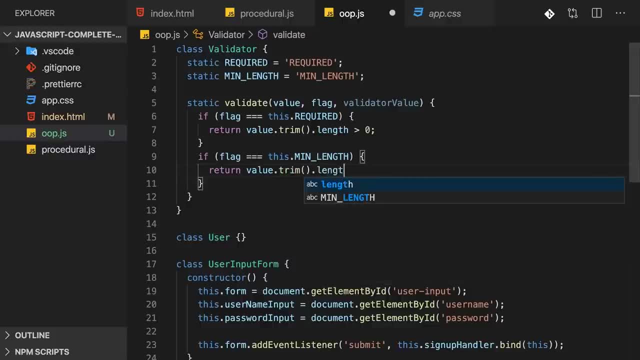 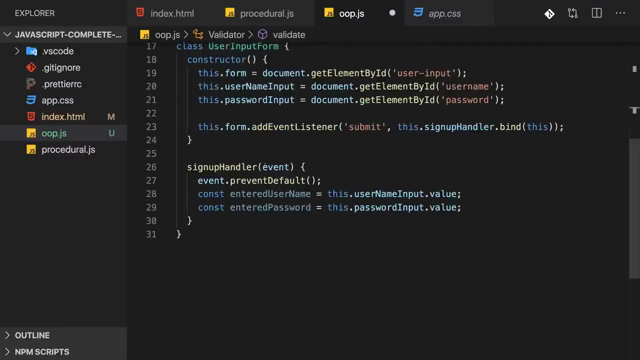 then I will return value: trim length, greater validator value. So this extra argument with which we can configure validation. Why am I doing it like this? Well, simply just to show that now we would have, we would have a reusable validate function, Because in the user input form, here in the signup handler, 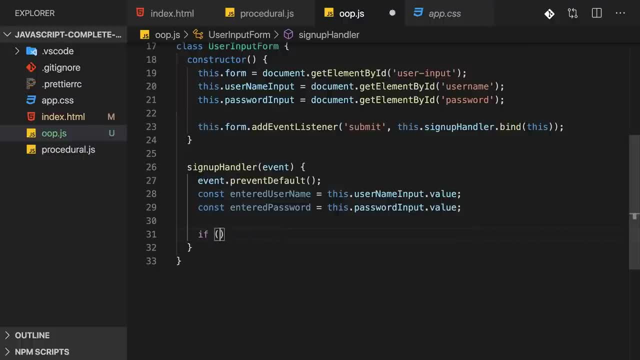 we can now use this. We can now simply check if validator. so this class I just worked in dot validate, which we can call like this because it's a static method, Hence we don't need to instantiate the class If this yields true for the entered username. 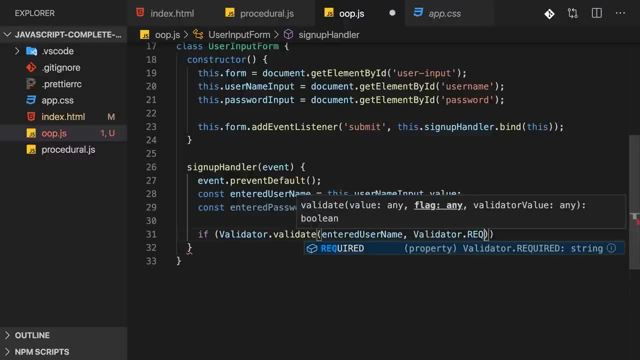 which is the value and validator dot required as a flag. So I want to validate this Here with the required validator and check if it's not empty. If this returns true, I'm fine. If it does not return true, indicated by this exclamation mark here: 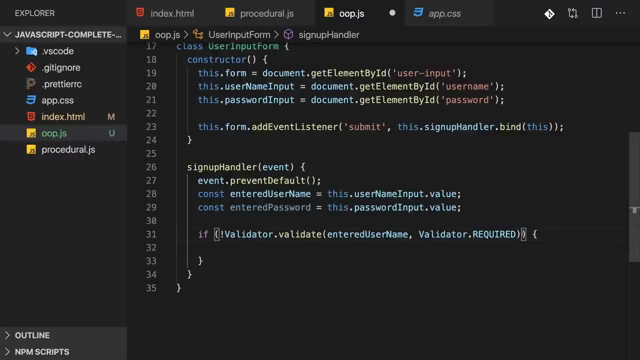 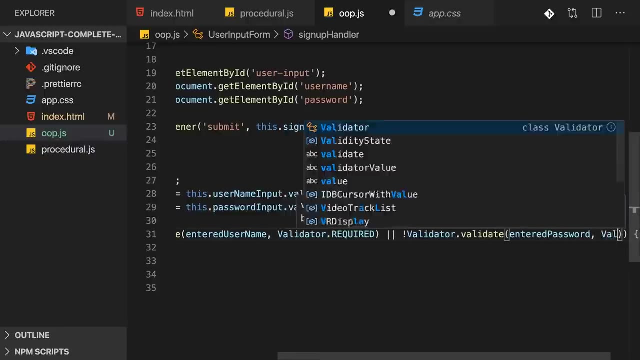 I want to show an error, but this is not the only validation, Of course. I also want to check one other validation logic here, One other expression, If not validator: validate for the entered password, for the min length flag And the value of five as a minimum length. 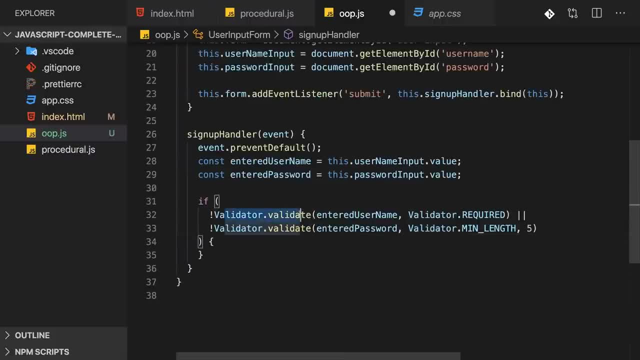 If this returns not true or this first one returns not true in any of these cases, I want to make it into this: if block- And here we can now show an alert and say invalid input- username or password is wrong, Password should be at least six characters. 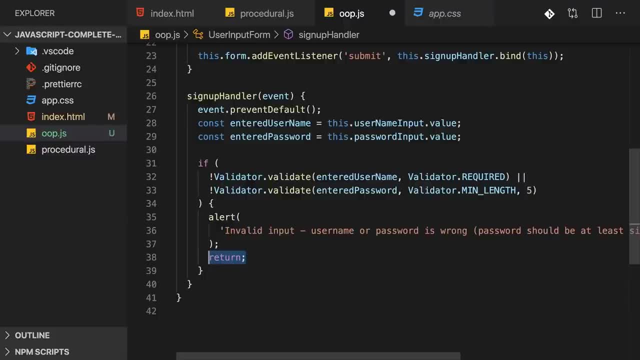 This is the alert we could show here, And then we want to return here to not continue with this method execution. So the error message, the error handling, still happens in this class here, which makes sense because this is the place where I do work with my concrete values. 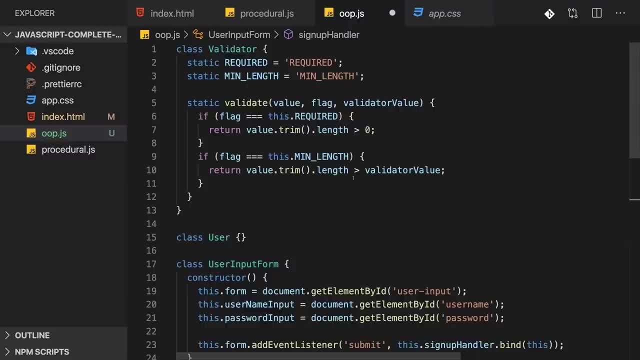 But the logic for checking the input is outsourced in a separate class. Now, this is not a must do, but it ensures that we could now reuse this validator in other forms of this application as well, And we might, of course, have more complex validation logic in there than we currently do. 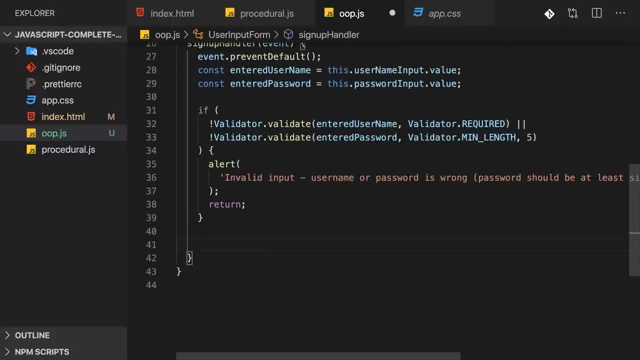 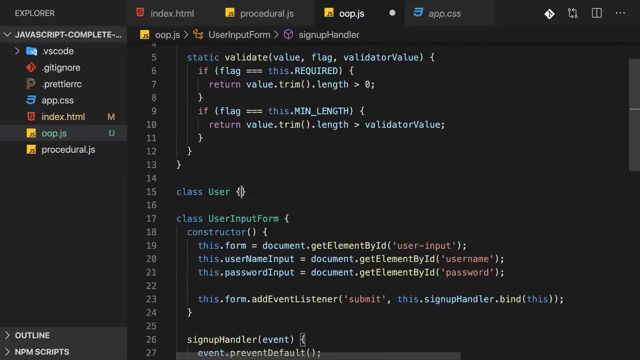 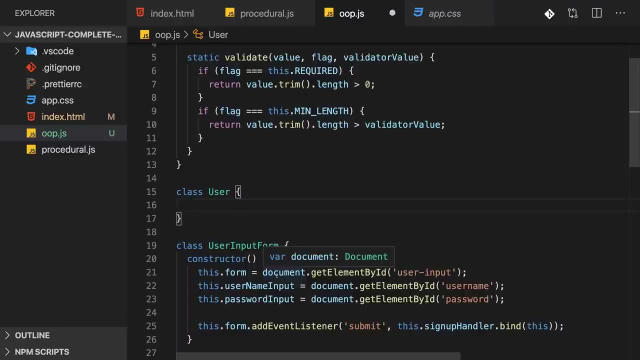 So now, with this, we know that after the save check, we have valid inputs And hence we could now create our new user. So for this, let's go to this user class and work on this. Here I want to define how a user should look like and attach any logic to it which it should have. 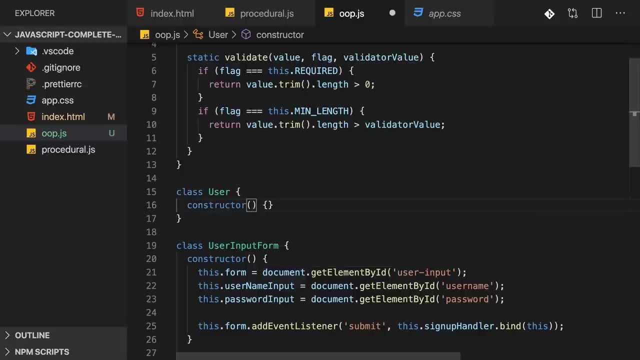 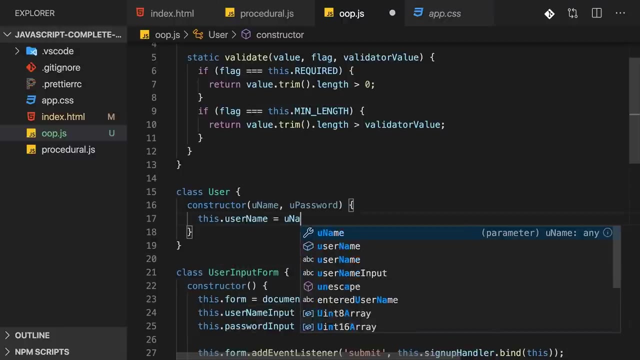 So, for example, here let's add a constructor to define some values with which we create a user, Specifically the user name And the user password. let's say: And then in here we have this user name- set it equal to you name. and this password, set it equal to you password. here. 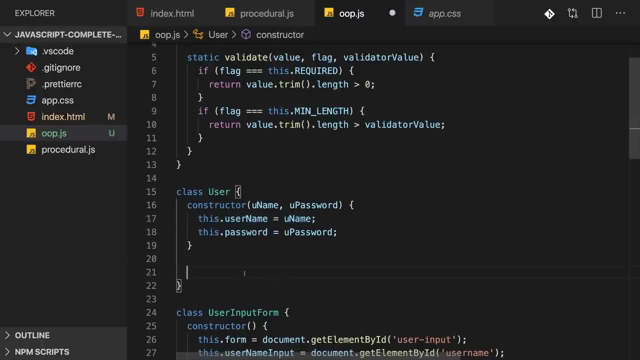 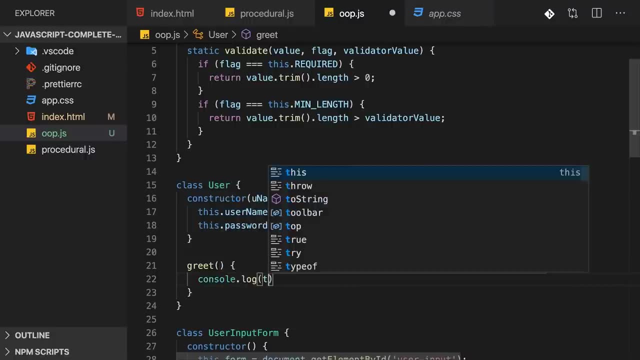 This would allow us to create a new object with these two properties. But I also want to add some logic. I'll add a greet method here to this user object where I just say: console log: hi, I am plus this user name. 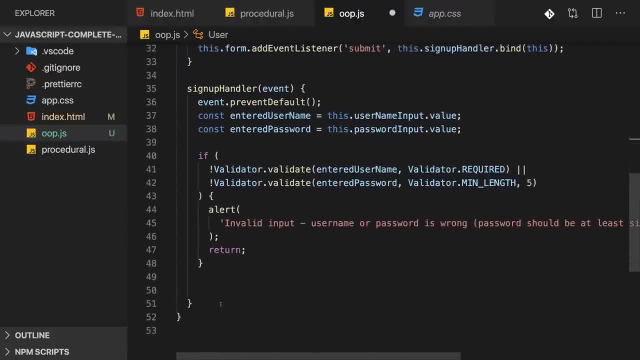 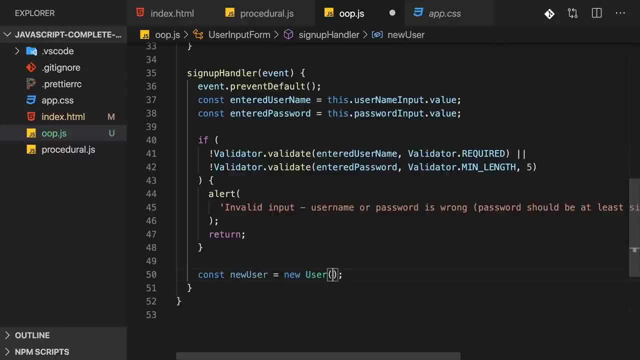 And with that we can create a new user Based on this class down there, our new user with new user. here we need a new keyword to construct a new instance of the user class And we forward our entered user name and our entered password here. 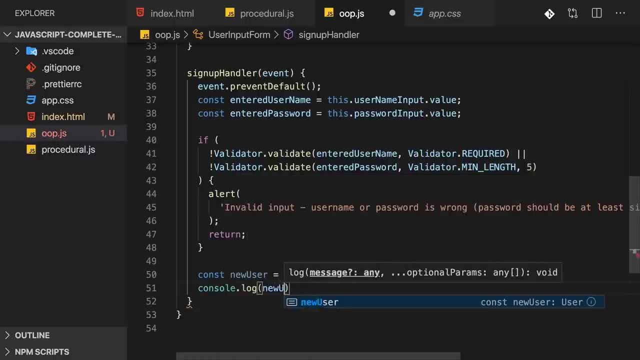 And thereafter we can not only log the new user but also call new user dot greet to execute that greet logic. And with all that done there's just one remaining thing now. Thus far All the logic lives in the user input form. 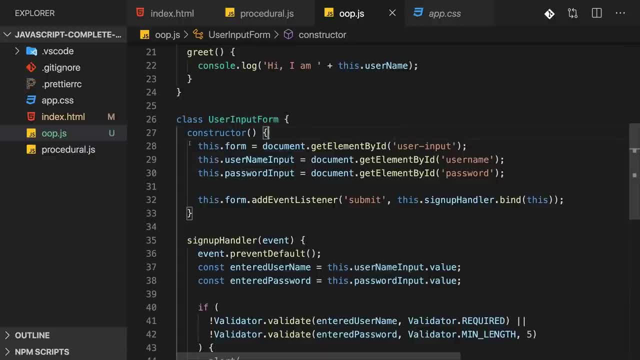 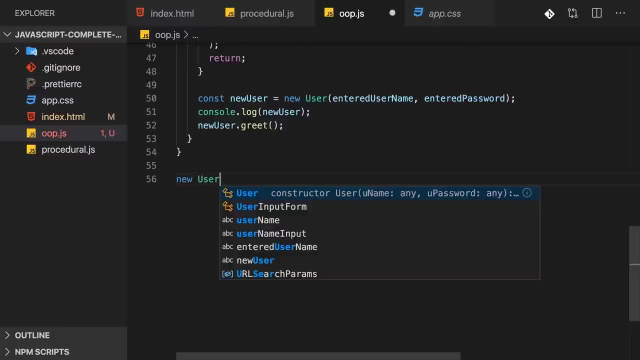 But this is just a class right. We need to instantiate it to bring this code to life. So below this here we can call new user input form like this to create a new instance. We could store it in a constant. But if we don't work with this constant, we also don't have to do that. 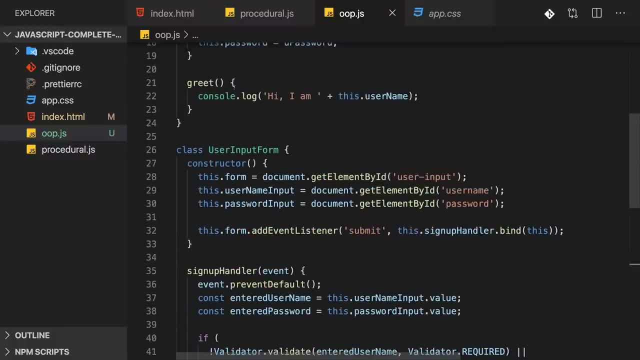 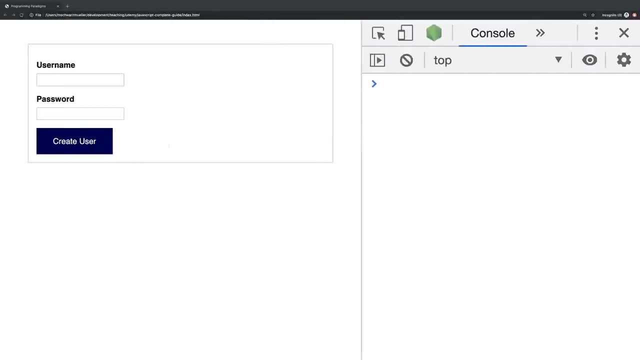 So here I'm just creating a new instance And with that this class here now comes to life. We run this constructor, We set up this event listener And we're there. We're good to go. So now, if we go back and we reload this page, if we submit an empty form, we should get an error. 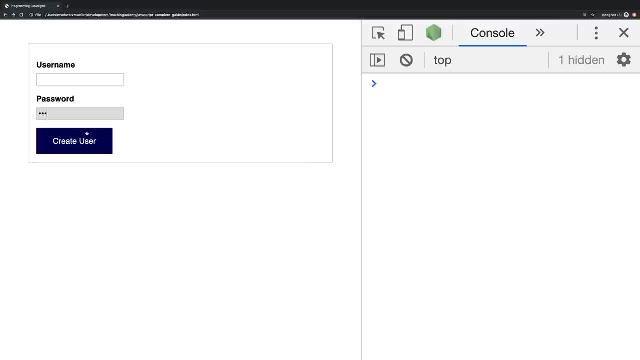 And indeed we do. If I enter a valid password here but I have an empty username, it still gets this error. And if I enter a valid username here but my password is too short, we still get an error here. If I enter a different password which is long enough, we do log our user object here and this greeting. 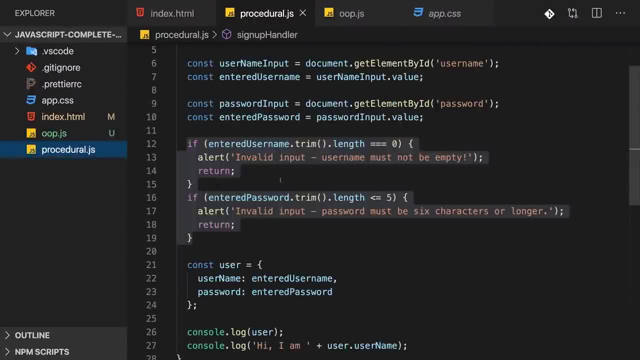 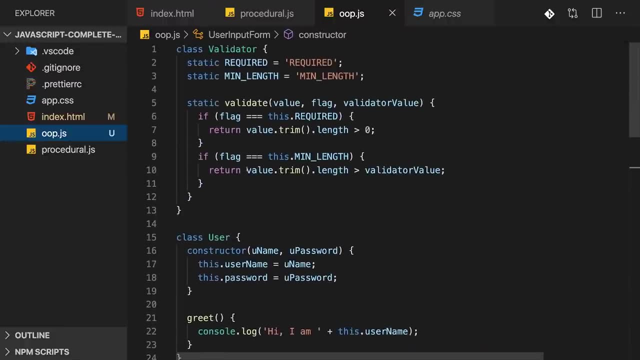 So this now works And it's essentially the same. It's the same logic as before in the procedural style. The difference is now that we think about our code as different objects working together And we split our code logically into entities, which can make it easier to reason about your code. 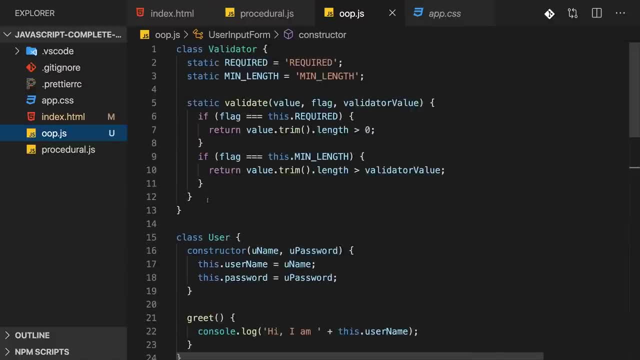 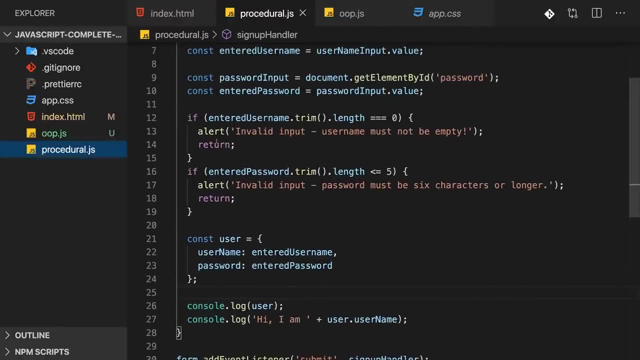 It can also help with reusing code, As I mentioned at the example of the validator, because we can use this anywhere in the application in the procedural style in the way we're doing it at the moment here. we would have to copy this around to share it. 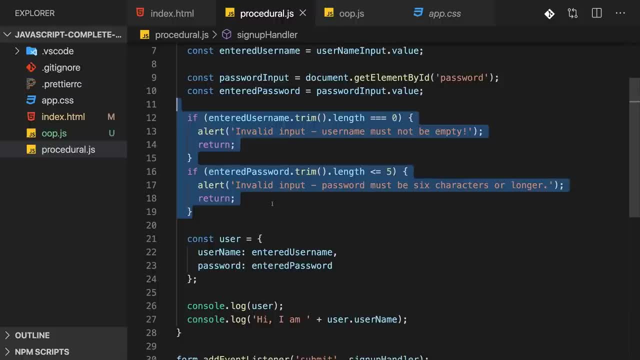 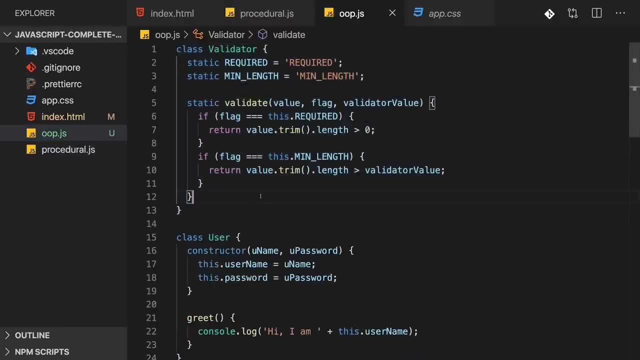 And again copy and pasting. It's bad because if you need to change your logic in one place, you then need to change it in 10 places, or how often you're using it. So that's the object oriented style. So, last but not least, let's explore the functional programming style for this. 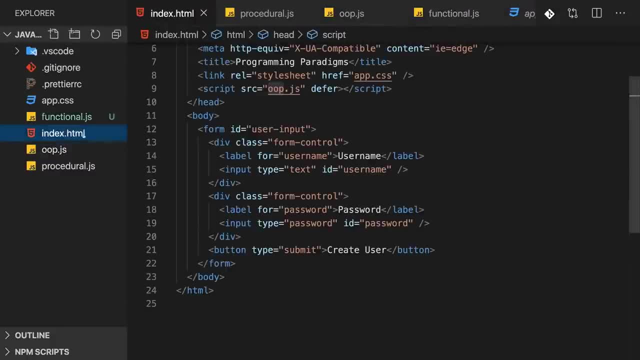 I'll create a new file here, functional dot JS, And, of course, import this year in the index HTML file functional. The idea behind functional programming now is that we organize our code around well functions so we can still then reuse And share logic by simply sharing a function, by exporting it and importing it in another file, and so on. 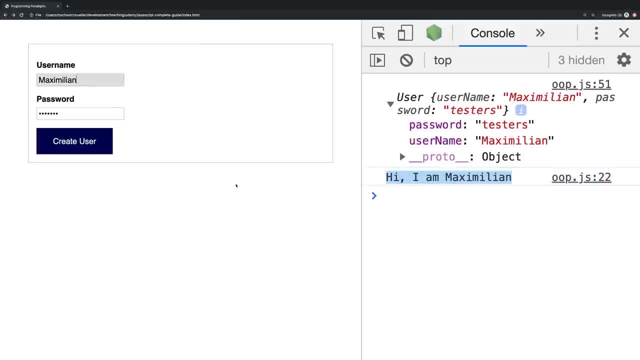 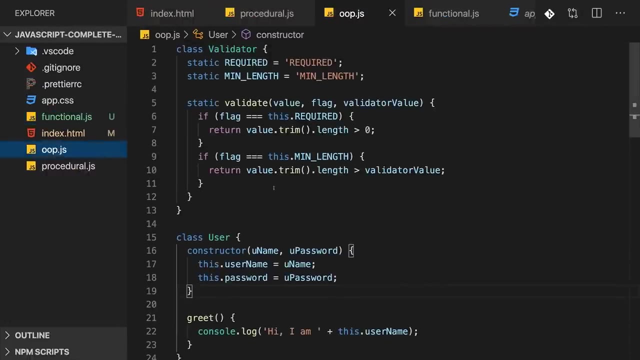 So how could we split this application here into a functionally written application? It can be hard to think about this if you're relatively new in programming. My personal experience shows that object oriented programming is relatively easy to pick up because it's close to the real world. 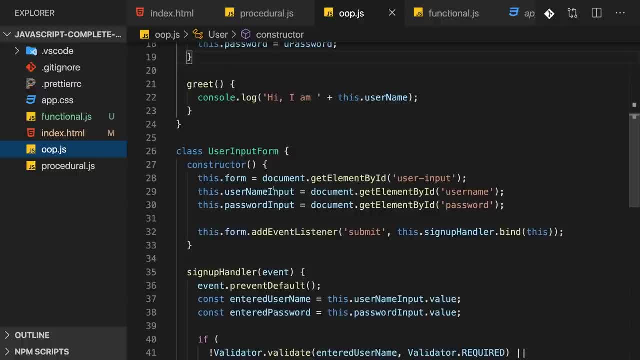 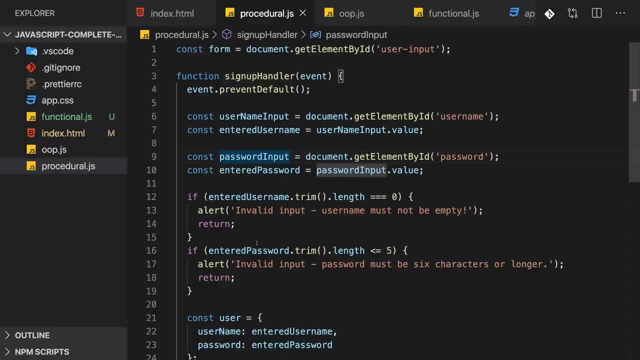 So to say, we think in objects, And that's how we think about the real world as well. The procedural style also is not too hard, because we execute code step by steps, And therefore all we have to do is that we have to think about what we want to do in our application step by step. 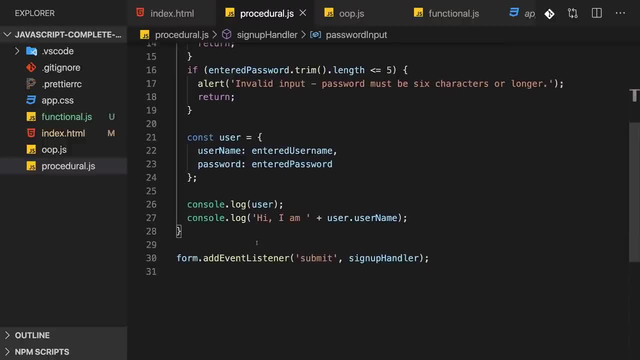 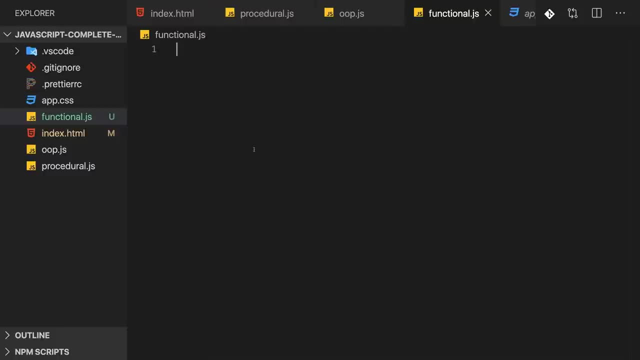 So what should happen when? and then this code is basically writing itself. Now, in the functional world it's a bit like in the object oriented world: We think about the different things that make up our application, But the things are now not. 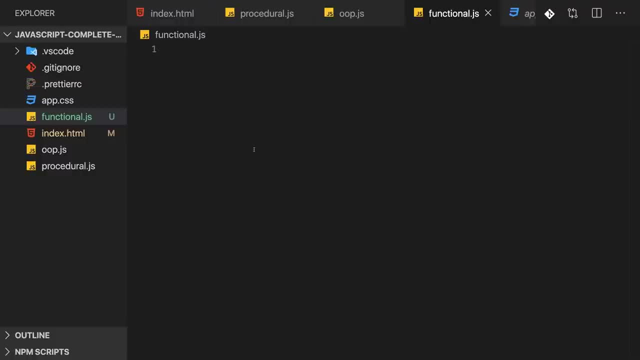 Objects, but instead different logical blocks, something like a validate function, a function to get access to a DOM element, a function to extract user input, a function to create a new user, a function to greet a user. So basically we try to split our code into the different logical blocks we have here. 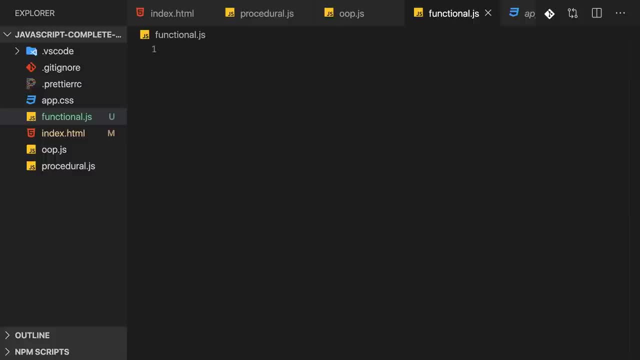 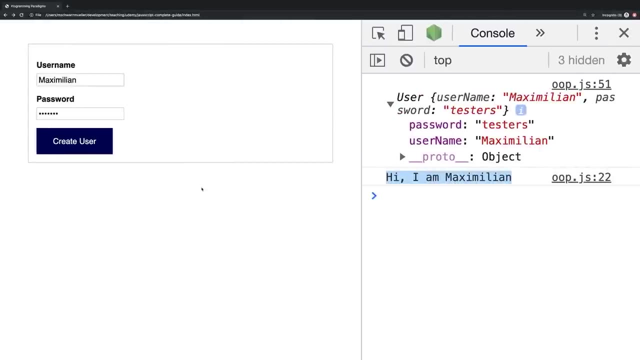 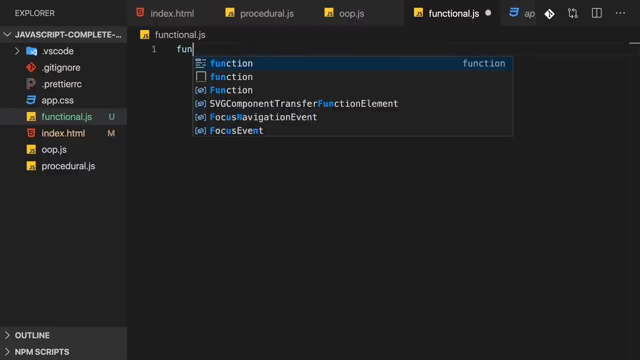 So in functional JS, how could we get started? Because maybe that helps us understand how it works- It still starts with us getting access to the form right. We need access to the form so that we can listen to the form submission. To get access here we could write a new function. 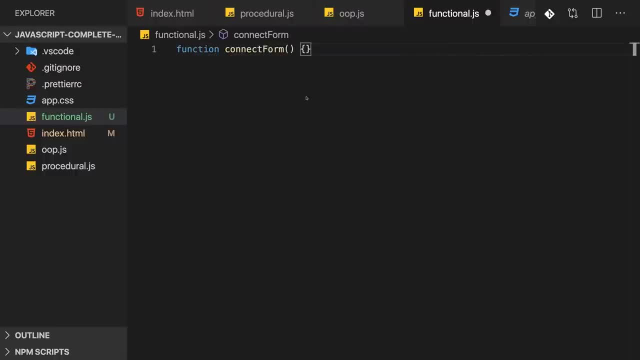 connect. form name is up to you And, by the way, you can write this function in any way you want In this function declaration style here. you could also write it as a function expression or, of course, you could use an arrow function here. 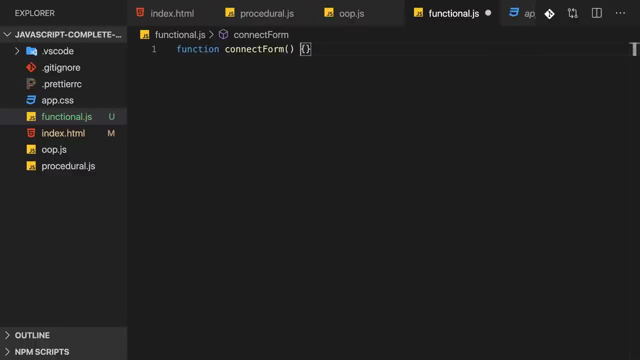 if you wanted to. that all works Here. I'll just write it like this. So connect form just like this, without any parameters for now And in there I want to get access to my form and I do so by calling document getElementById- user-input. 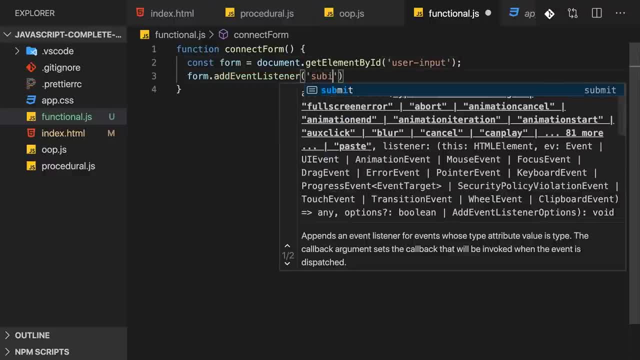 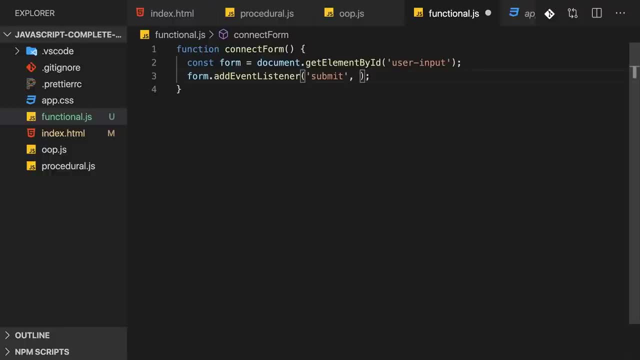 And thereafter I will reach out to my form and add a submit event listener here. And then then what? Then I want to point at a function that should execute when the form is submitted. So maybe let's add a new function here. 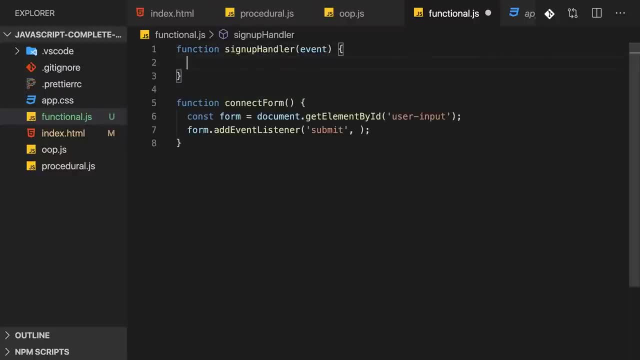 The signup handler, which gets this event object, which calls event prevent default. It will also do more than that, but this is something we definitely need to do, And then I pointed it here- This is something we could do, but it's not the perfect way of setting this up. 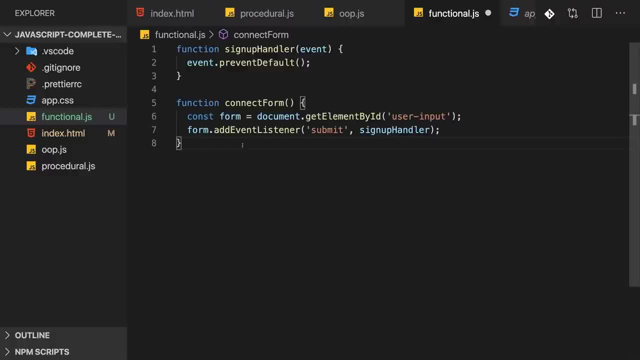 Instead, the idea or the core philosophy you really should embrace when writing functional code is that your functions should be pure and all the data they work with is received as parameters, So that your functions are as predictable and reusable as possible. So for this, connect form function. 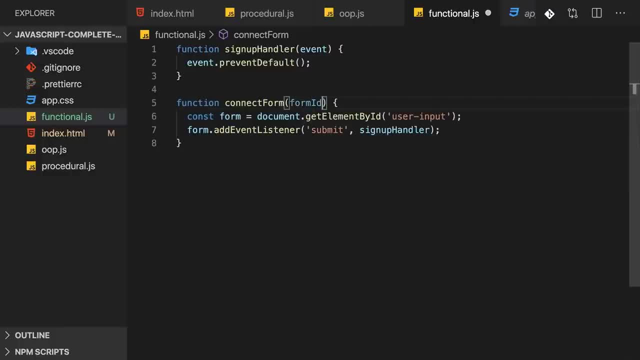 this means that we would probably get the form ID as a parameter and also the form submit handler function as a parameter, And then here, instead of pointing at user input, here we would point at form ID And here we would just say form submit handler. 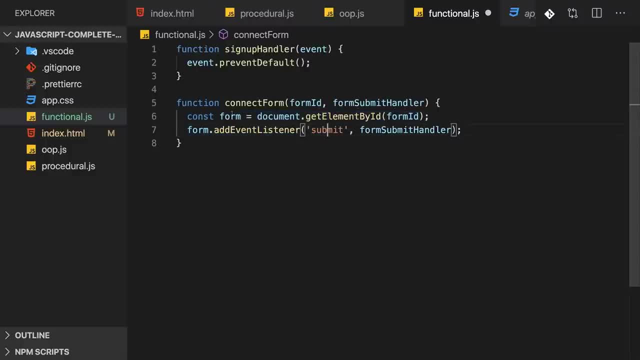 And now this function has code which is totally reusable, which makes no assumptions about what's in your HTML file. It makes no assumption about this ID and about the name of the function that should handle the submission. Instead, we would call connect form here. 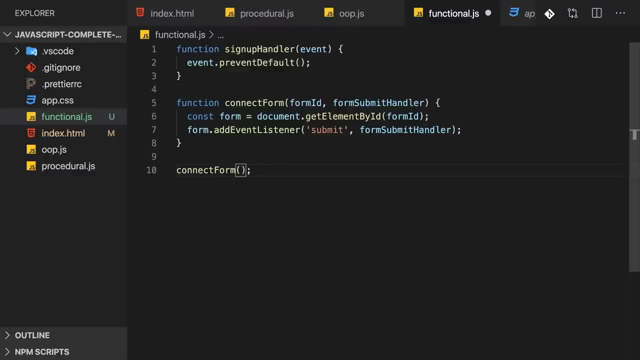 when our app is initialized, So when this JavaScript file is parsed and executed for the first time, And here I would feed in the concrete values, So user input and a pointer at signup handler. Now, of course, in this simple app, 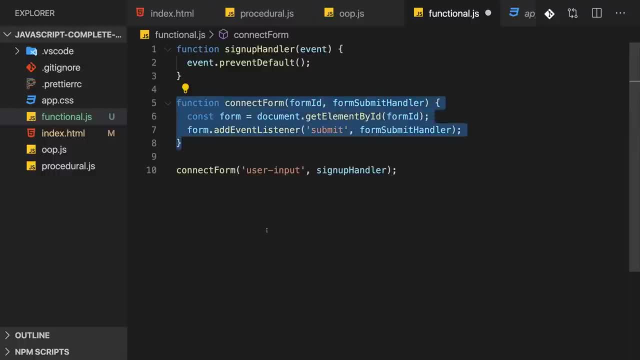 we don't gain much by this, but now we really have a function which is pretty focused, pretty straightforward, pretty easy to understand and which is also pretty reusable because it's not tied to a specific form in the HTML code. If we had multiple forms, 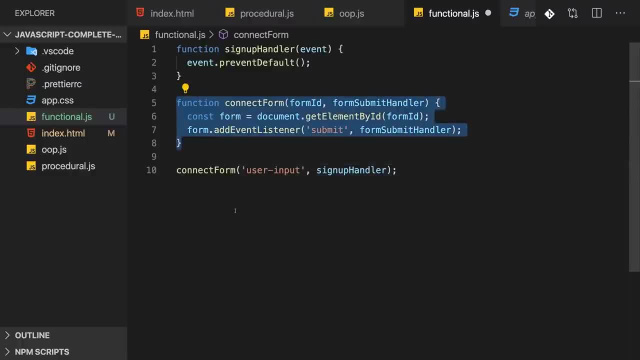 which we wanted to connect with submit handlers. we could reuse this function and we could just call it with different arguments. That already is how you should think about code when thinking in a functional programming style. So now we connect this form, we point at the signup handler when the form gets submitted. 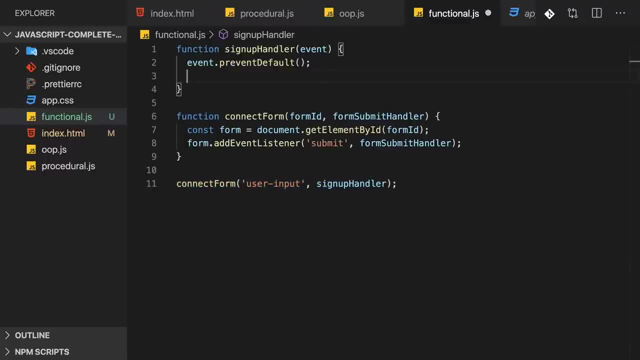 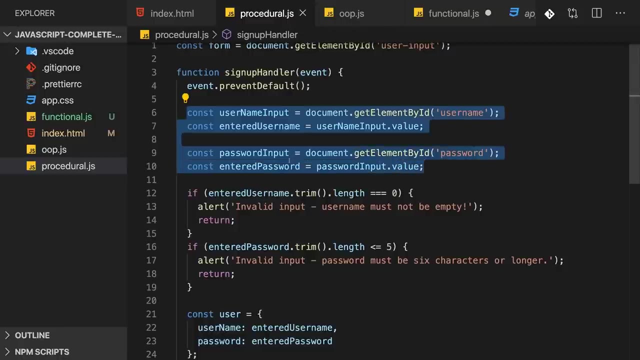 In the signup handler. we now want to get our user input and we now also, of course, then want to validate it and create a new user. Now again, we could copy our logic from procedural right. We could copy this logic here for getting the user input for the moment. 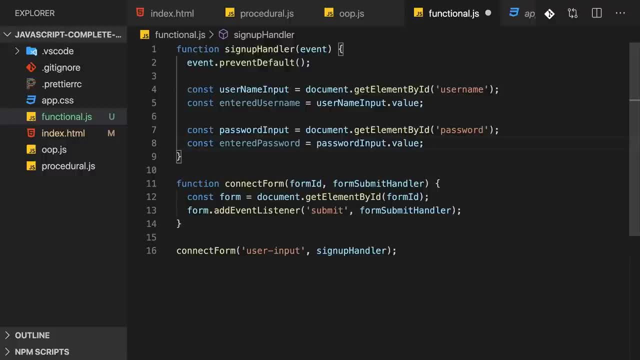 and paste it in here, And this would work, but we're not really thinking in a functional way. Let me just show you What did I just say about functions. Well, they should be pure and should receive all the inputs they need as parameters. 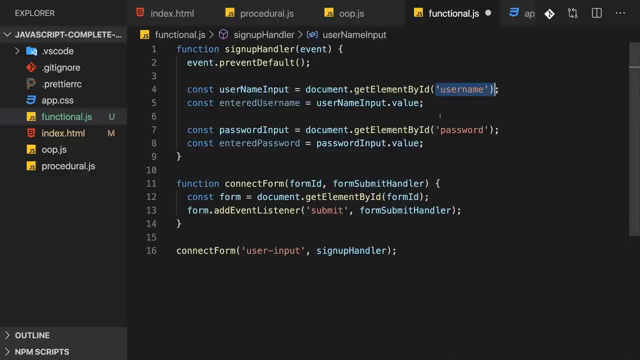 And here again I'm hard coding IDs, which are IDs from my HTML document, into the function. Now, we could do this, but is this good? Well, it's certainly not bad. Now you might argue that hard coding these IDs into the function is not something you wanna do. 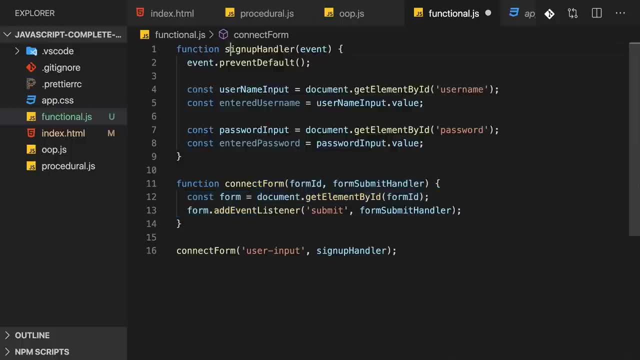 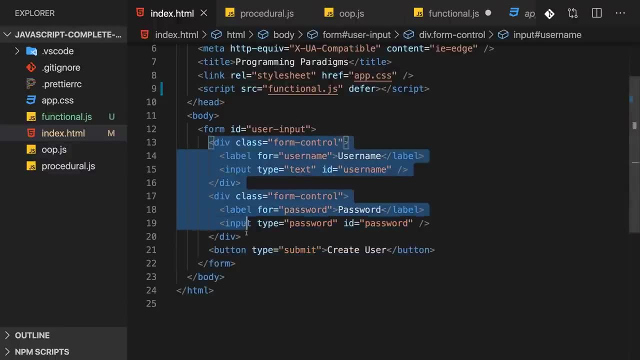 because we got rid of it here. But I would argue that the signup handler is of course a very specific function, which indeed can be tied to the HTML file, because it really is about this signup form. It's not a general function here, like connect form was, which should work with any form. 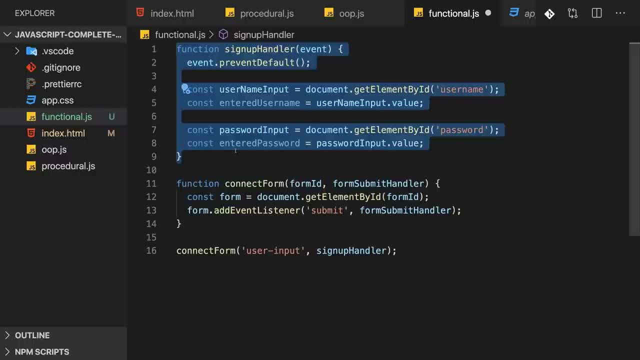 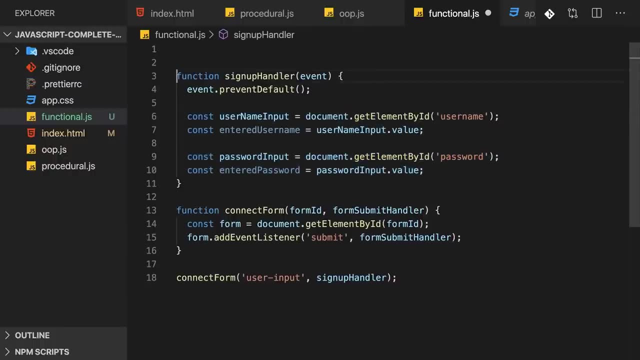 This really should only work with the signing up logic. So that is fine, But we're basically having some code repetition here. Why don't we create a new function here which we name getUserInput? And here I have, I expect to get my input element ID. 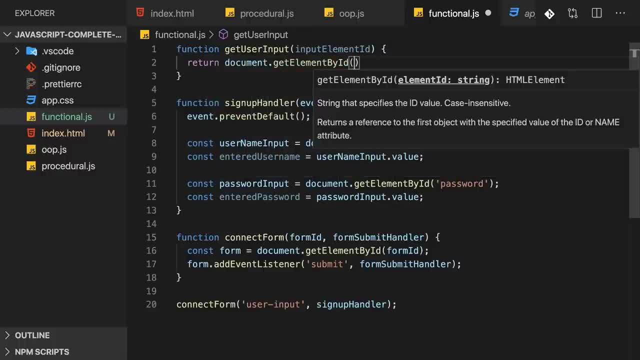 And in this function we then return document getElementById, to which I forward the input element ID parameter, And then I access dot value here. Now, of course, this only works with input elements, but that's the idea behind this function. 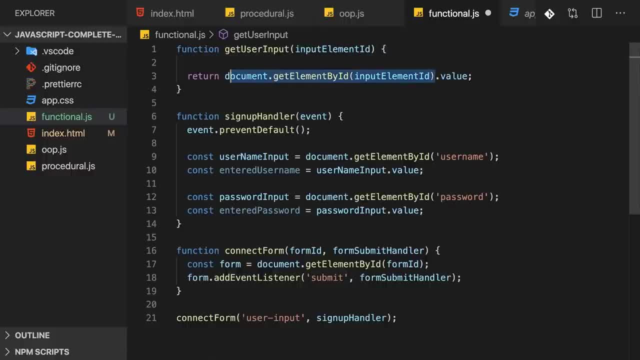 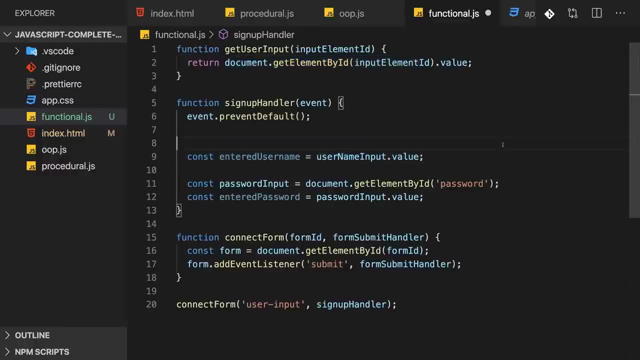 So we could add an extra check which checks if this is an HTML input element, but here I just assume that it always will be one, And now we can rewrite this. We can get rid of this line here And entered username now simply is getUserInput. 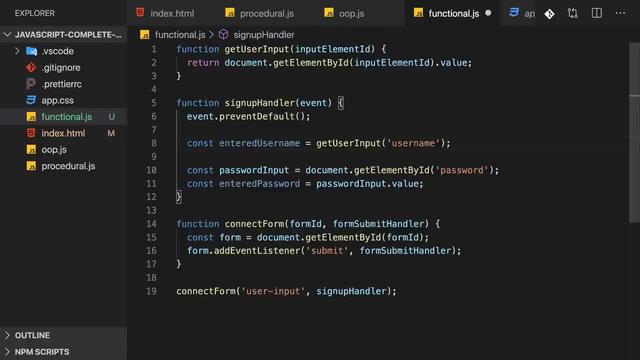 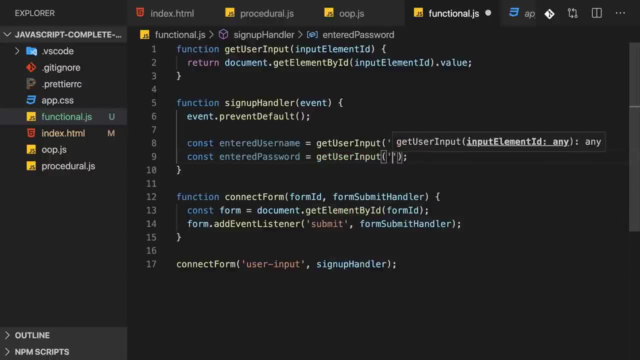 for the username ID And we can get rid of this line And the entered password now just is getUserInput for password, And again we have a reusable function here and this is now leaner and more focused. So now we got the input. 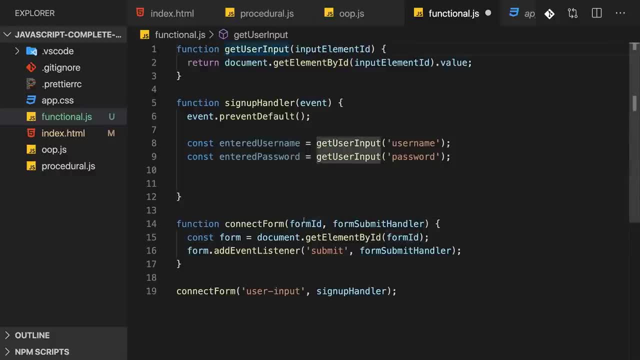 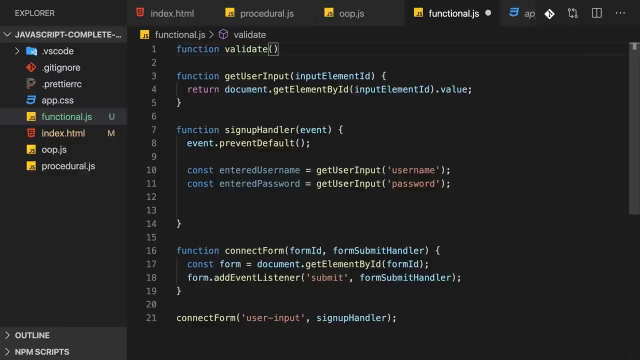 Of course we want to validate it. So unsurprisingly, we create a new function. So unsurprisingly, we create a new function. So unsurprisingly, we create a new function for this, the validate function. And here we could again follow the logic we set up. 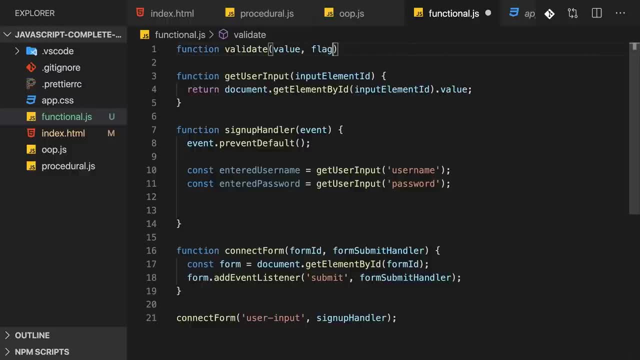 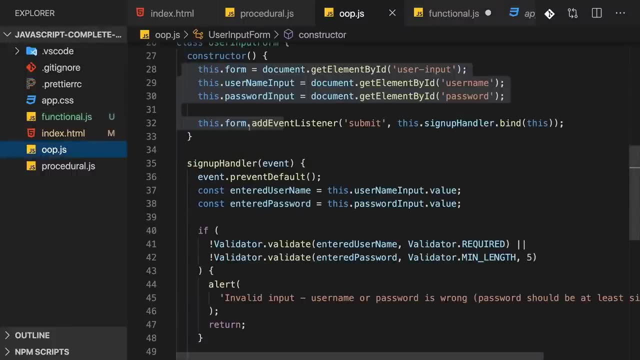 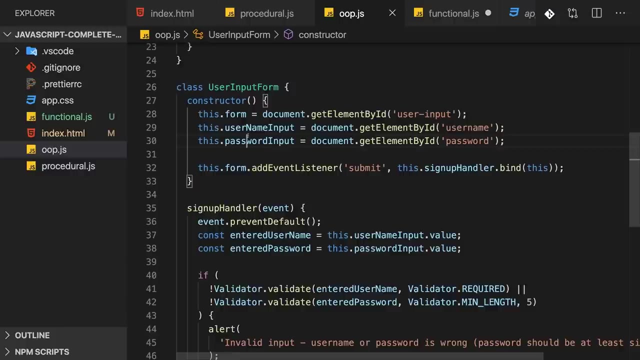 in the object-oriented part. We can expect a value, a flag and a validator value here And then basically copy over the logic from OOP, because object-oriented programming and functional program is not that far apart. It's a bit more than just translating classes to functions. 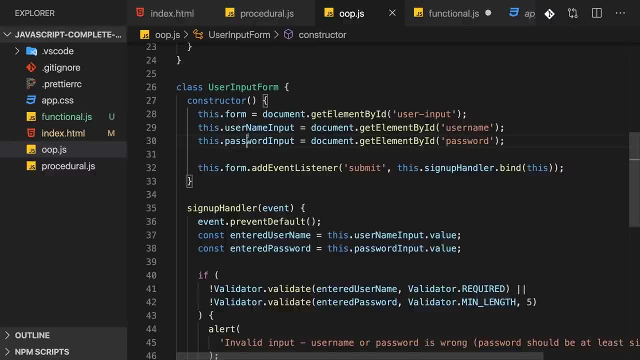 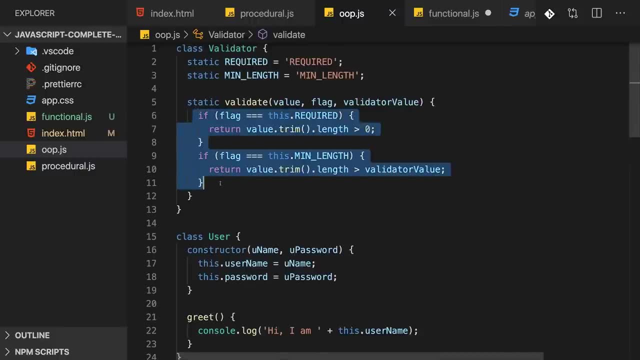 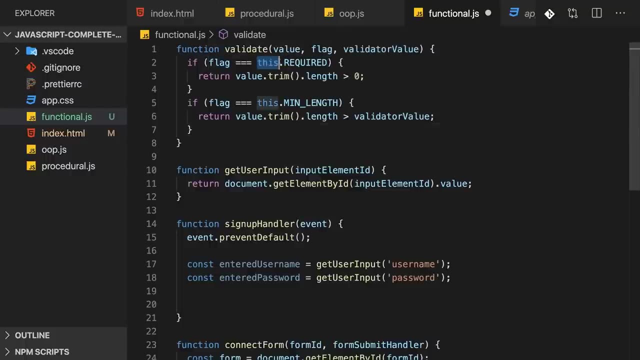 but the idea of organizing logic in methods and in classes is not that far away from the idea of organizing logic in functions. So, unsurprisingly, we can copy the logic from the validate method here and add it in the validate function here. Now we just need to replace this required. 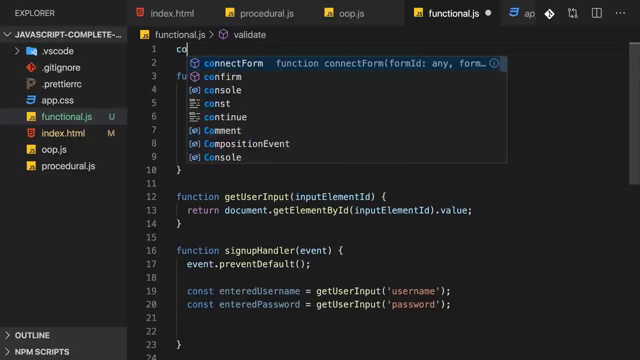 and this minLength with just required and minLength, and add some global constants here. And yes, this is also possible. Not everything has to be inside of a function. Not everything has to be inside of a function. Here we want some global flags, some global identifiers. 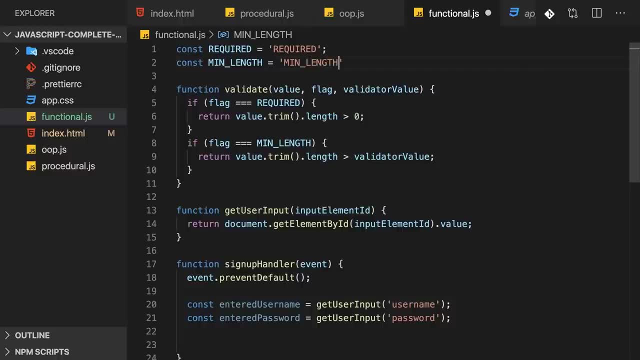 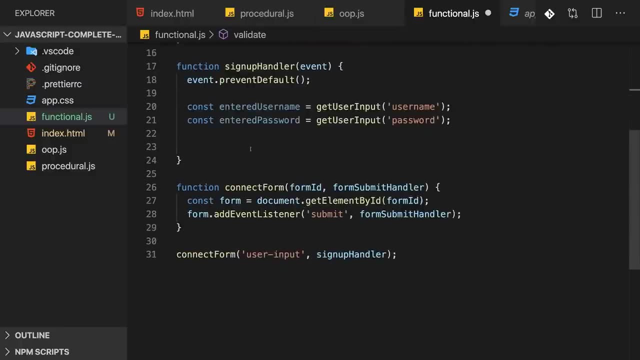 and therefore we can define them just like this in our script here. So now we have that, we have our validate function, We can now use this validate function here in the signup handler. So here we could now call validate and forward the entered username and so on. 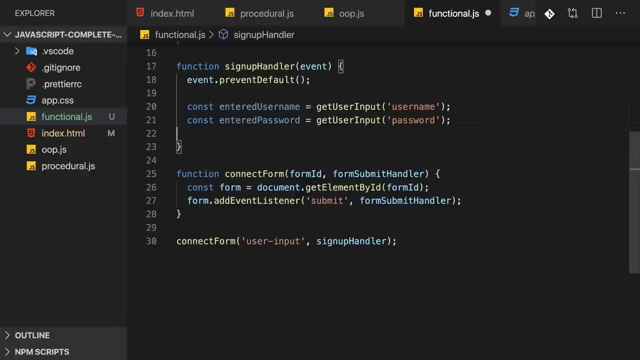 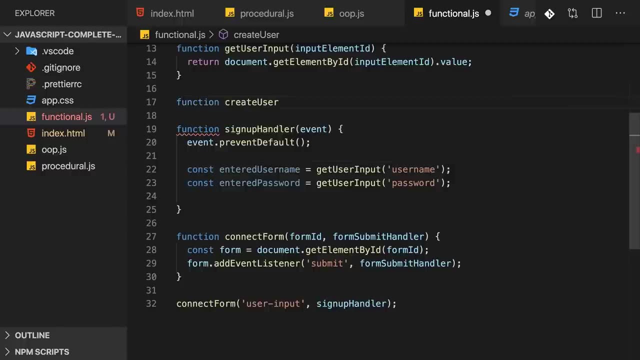 And that, again, would not be wrong. but I want to create yet another new function, maybe here, which I'll name createUser, And this is a function that takes the username and the user password And this should now run the validation, And that's just, of course, one way of doing it. 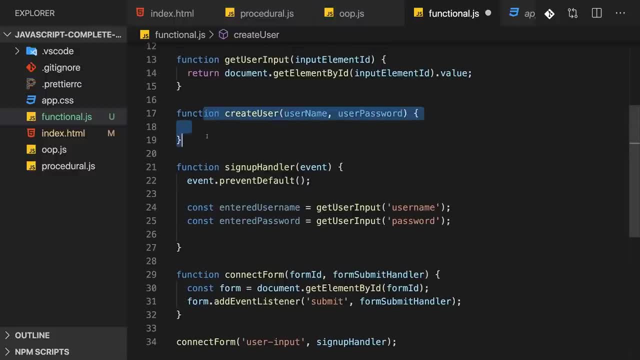 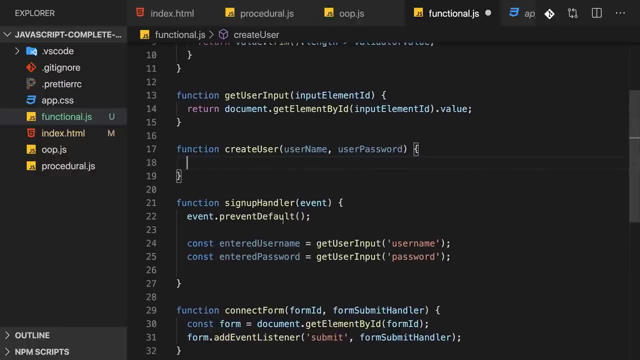 not the only correct one, just one way of doing it. So I want to run validation here And then, if it succeeds, also create my user. So in here I will now check if not validate for username and the required flag. So if this yield's false, 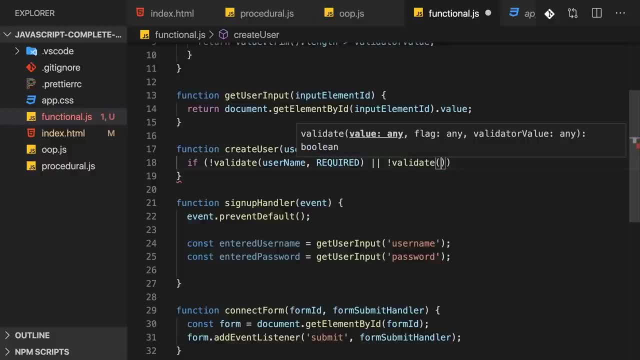 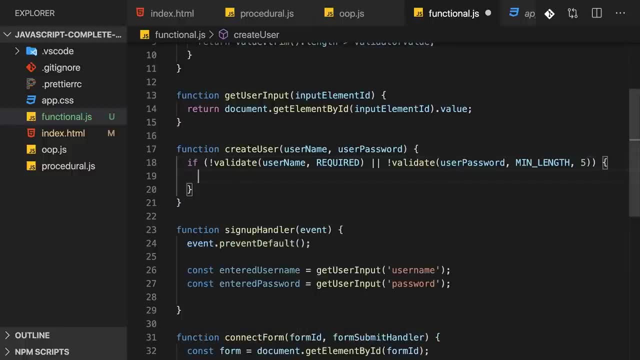 or if validate for the user password and the min length flag and a min length of five. if either of the two yields false, we could throw an alert, but this would be a side effect. Now, what's a side effect? A side effect, basically, is some logic you execute. 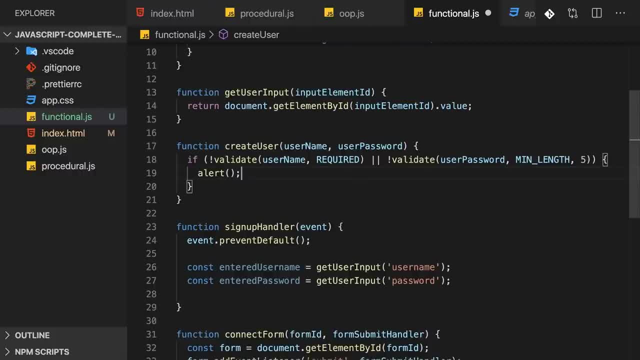 inside of a function which does something, outside of the function which sends an HTTP request which changes something, And the DOM or, like in this case, which shows an alert. So these are typical side effects. A pure function just receives parameters. 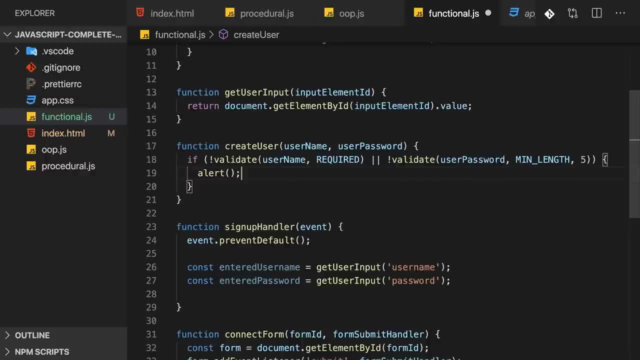 and then maybe returns something, And for the same parameters it always returns the same thing. An impure function which has a side effect might also do that. It might also return always the same thing, but it also might manipulate something outside of the function. 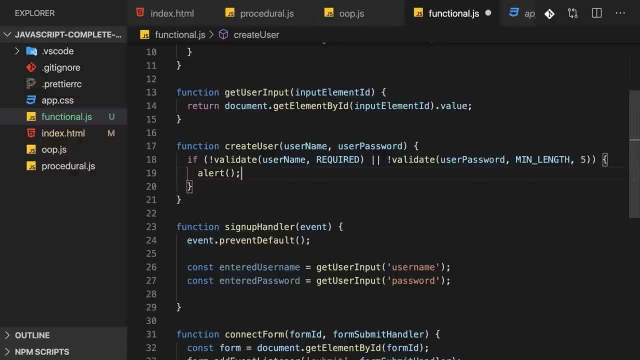 So, like I said, in the DOM, or send the HTTP request Now, sometimes you can't avoid this, but here I want to have create user as a pure function, So I will not throw my alert here. Instead I will throw a new error here. 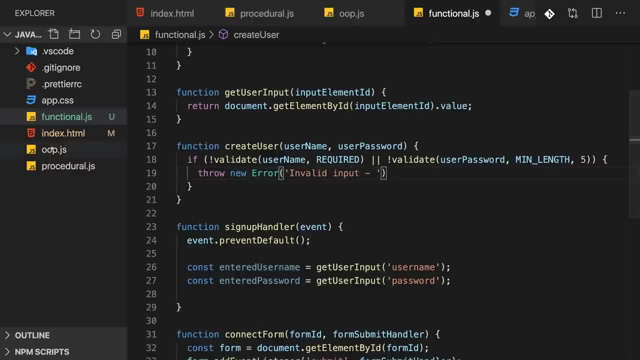 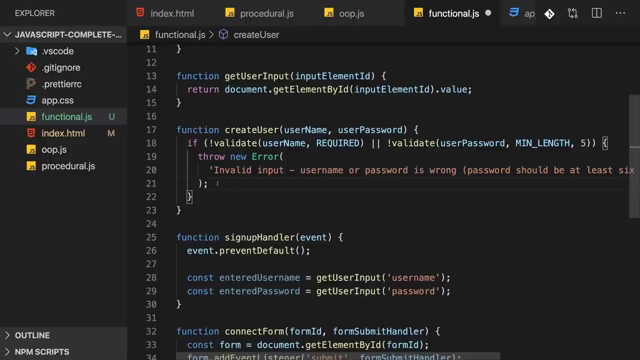 with an error message of invalid input, And I'll just copy the error message from the OOP file here. So copy that string and throw this here as an error message on this JavaScript error. So here we're not showing an alert, we're really throwing an error. 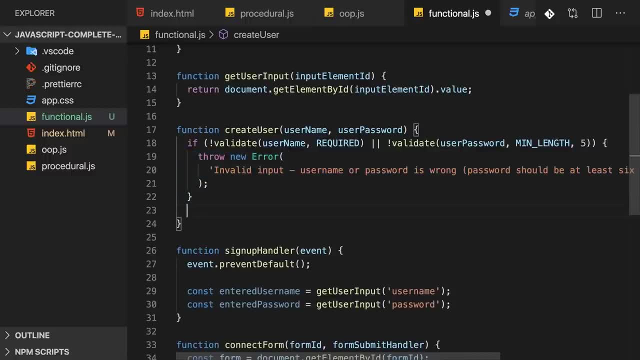 and that will automatically cancel the execution of the remaining function If this error gets not thrown. so if we make it past this, if check, if we do have valid inputs, then I will return a new object And that is my user with a username. 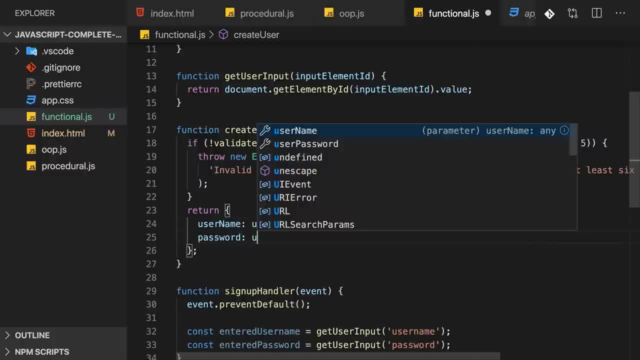 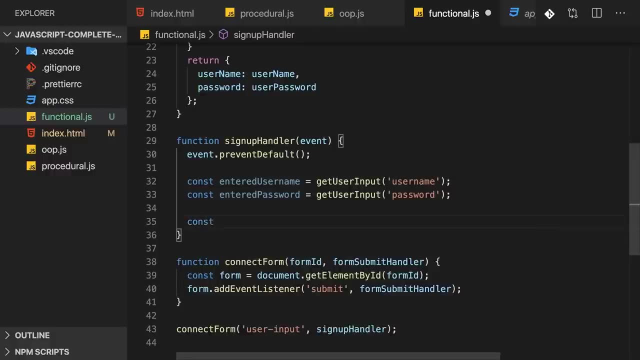 which holds the username value and with a password which holds this user password value. So now create user is something we could call here in the signup handler. We got our new user by calling create user and we forward the entered username And the entered password. 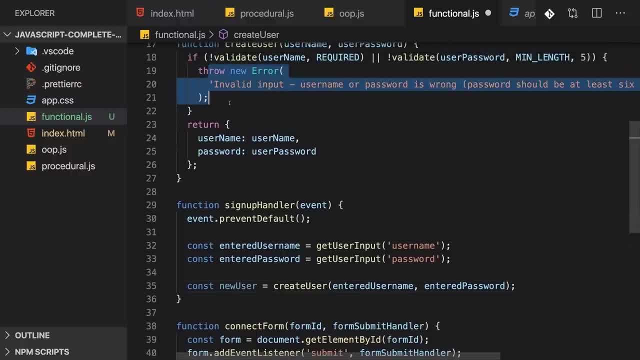 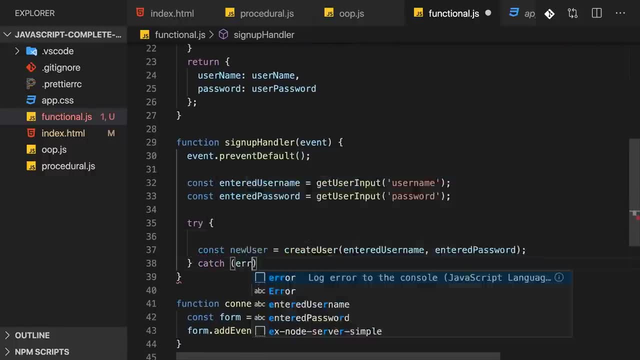 Now this could fail. however, This would throw an error if we have invalid inputs. So here we can use try catch. And again, we could use try catch in the object oriented style and the procedural style as well. Don't get me wrong. 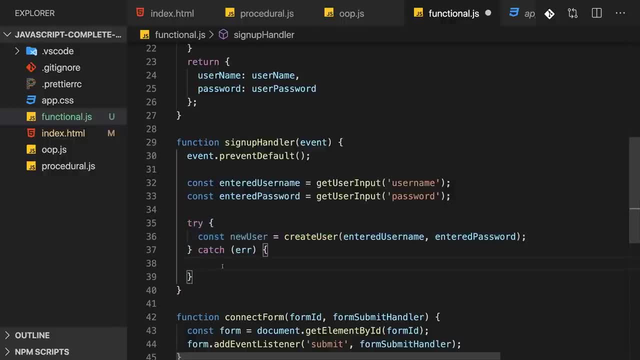 But now I think here is really clean to do it like this: We use try catch and we try to create a new user, But if this fails, I will now show my alert here And, yes, this will now produce a side effect. 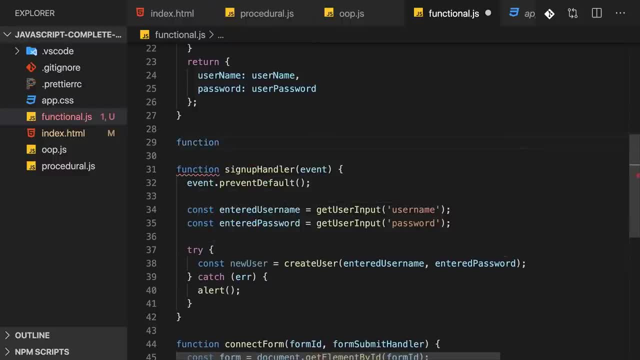 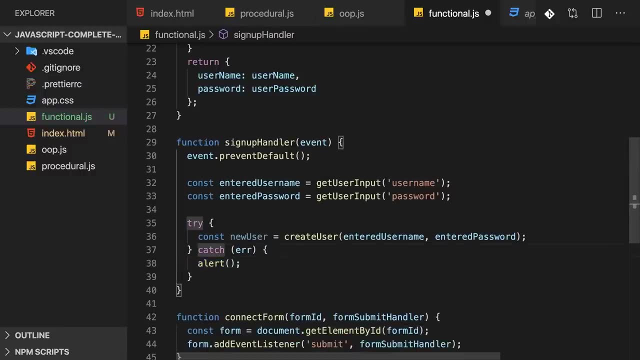 But we could even outsource this into a separate function: Show alert. But since I would do nothing else in there but call the alert function, I'll do it just in here. And, as I said, sometimes you can't avoid it. It's okay to have functions that produce side effects. 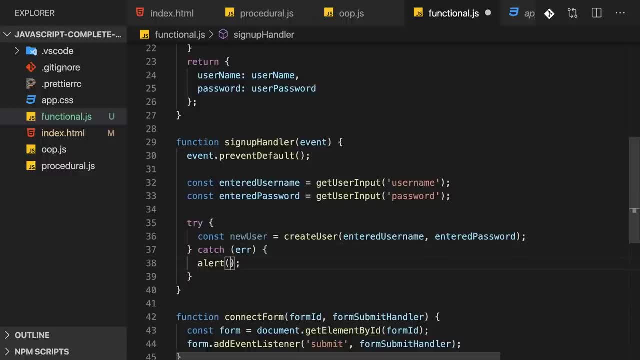 You just want to keep most functions pure and side effect free Here. however, I will output the error message in an alert. If this succeeds, however, I want to console, log the new user And, of course, also greet the new user. 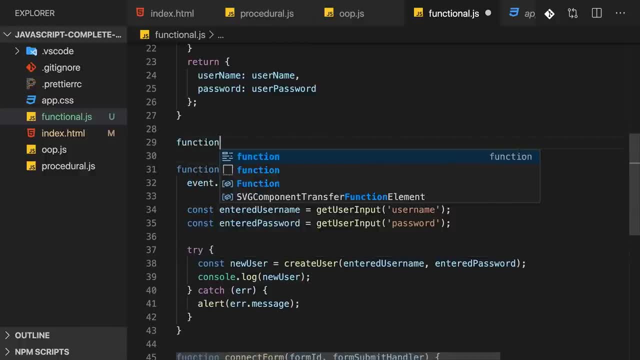 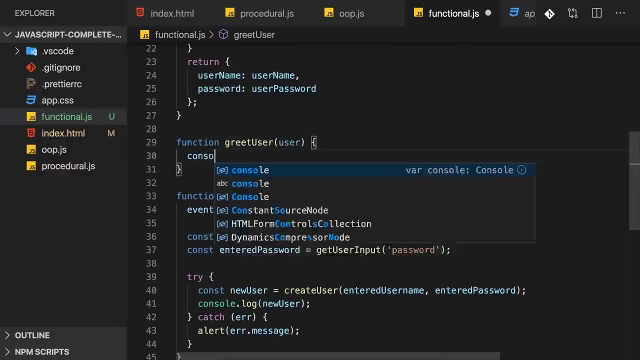 And for that we could create a never a new function here, the greet user function, which gets a user object and just calls console log: hi, I am. plus user username. And again, this here would also technically be a side effect. 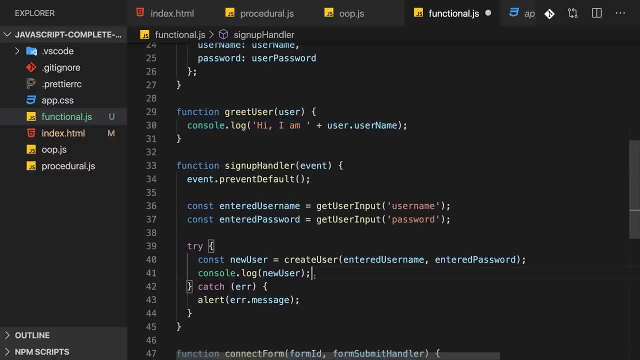 by the way, because we do something outside of the function. So here I can then call greet, Here I can then call greet user and forward the new user, And there are different ways of writing this. These are just examples, of course. 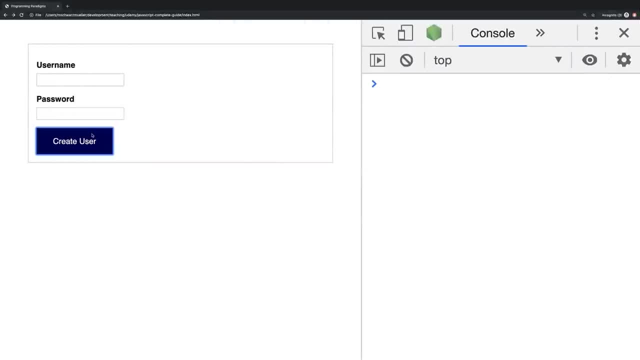 If we now save this and we reload this page. if the form is empty and I click submit, I get this error. If I have a valid username but my password is too short, I get an error If my password is long enough but the username is empty. 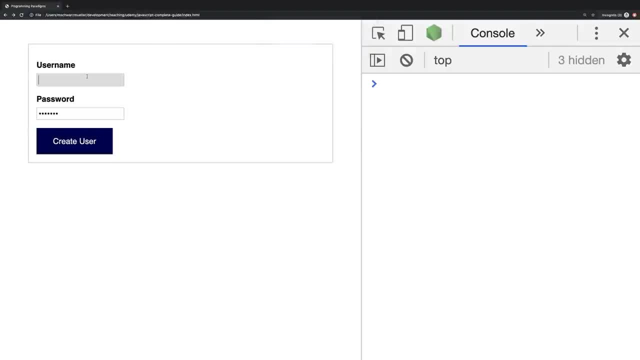 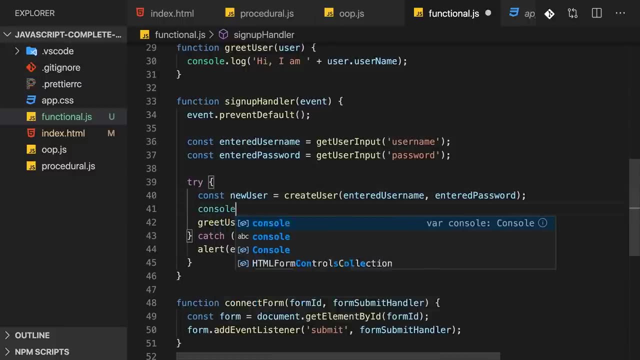 I get an error, And if both is valid and we click create user, we're showing: hi, I am Maximilian. The log is missing because I didn't enter it here, So here, of course, I want to log my new user. 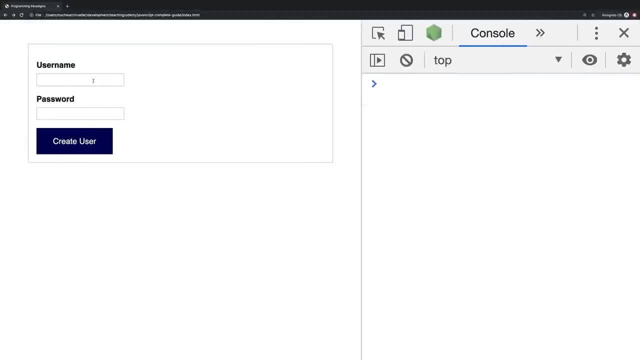 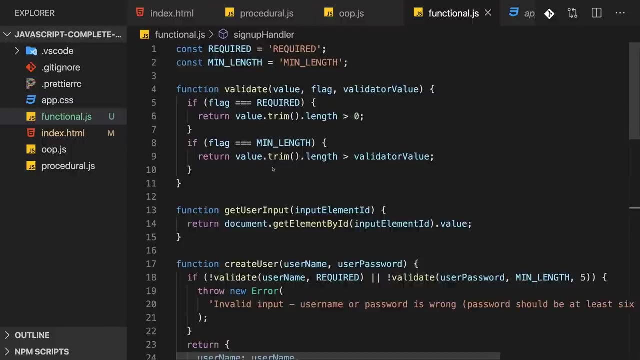 and then retry this. so reload, Enter the values here again, And now we get the same output as before. So this now really is working. And now this is an example of functional programming, The core idea, of course, being that we organize. 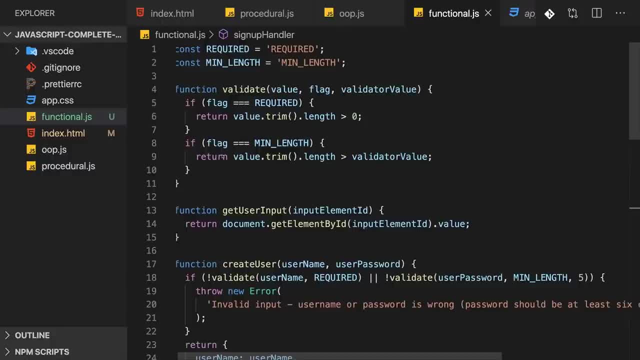 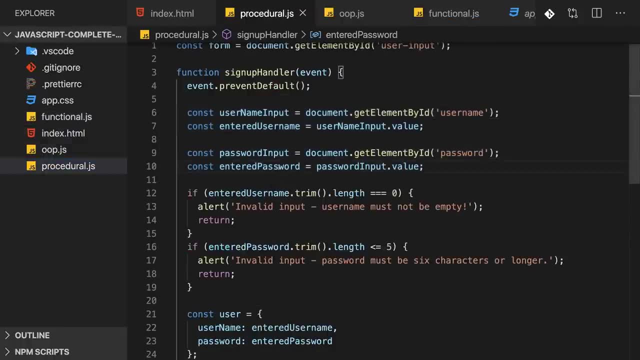 our code into functions, where most functions are pure and side effect free and therefore highly reusable. So we saw three different styles And of course you can also mix these styles. You could have a procedural style, where you also work with classes and where you have multiple functions. 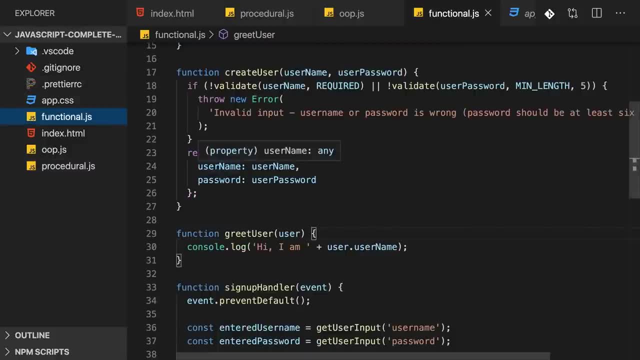 You can have a functional style where you somehow also sneak in some classes, though it then technically wouldn't be a pure functional style anymore. Which style is the best, though? Well, The best style is the style which best works for you. That really is the truth. 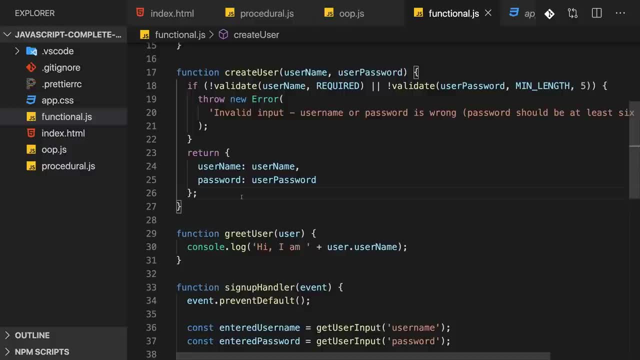 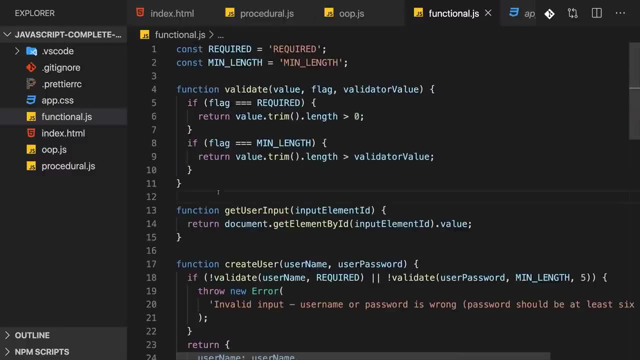 Now there will be people who strongly disagree because, like a couple of other things in programming, this really is something where you can have religious debates. You can really discuss this And for a lot of people it seems to be the most important thing in life. 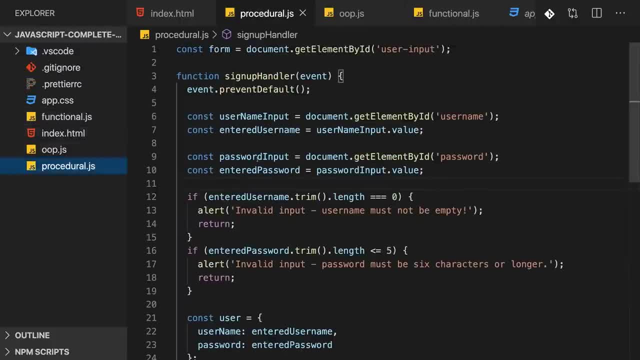 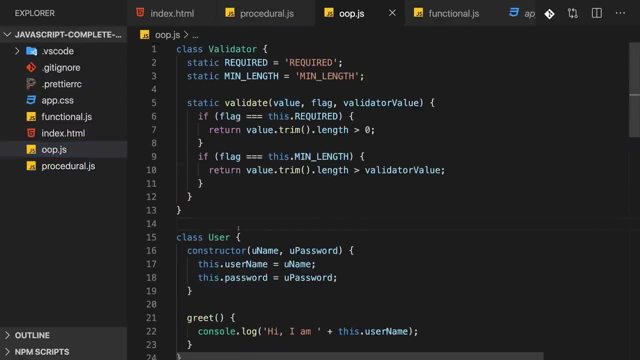 Not to me, though. You can write code, You can write apps with either style, And you should find the style that best suits your needs. Now, the more experience you get as a developer, the more you will see that, for certain application types, 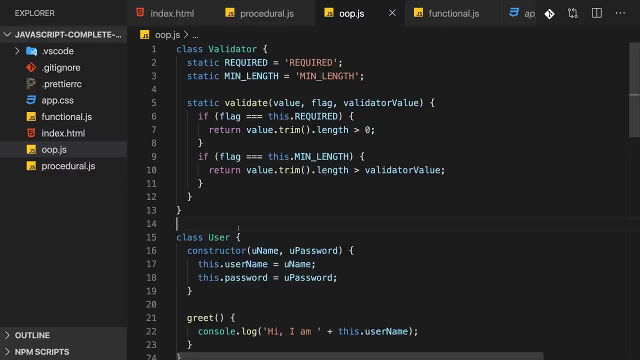 some styles tend to work better than other styles And again you can find discussions about this on the internet. Some of them are even kind of friendly, which will show different applications and different examples for when to use which style. You also sometimes have programming languages. 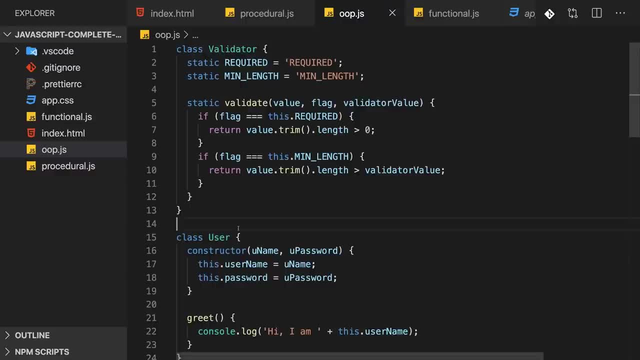 which strongly favor one style over another. For example, C Sharp is a programming language which is heavily object-oriented. JavaScript, on the other hand, is pretty versatile. There you can follow any style, And therefore sometimes you also are forced into a certain style, and sometimes you are not. 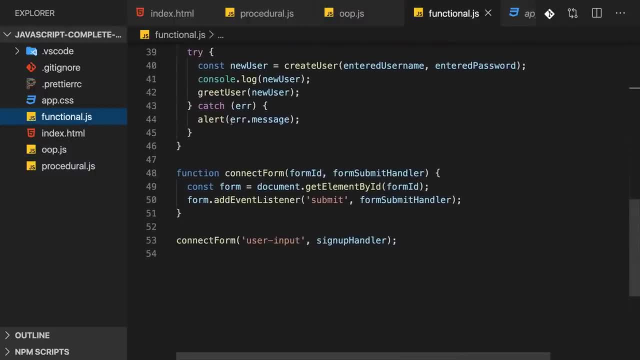 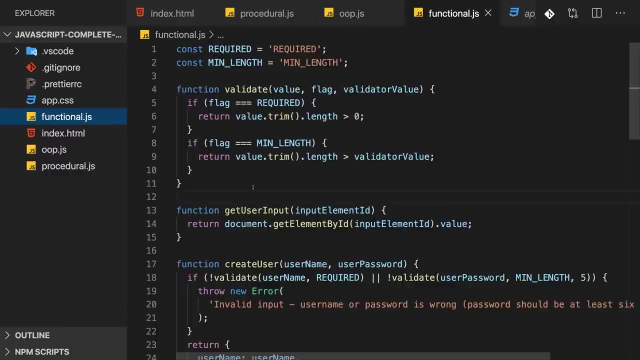 It's important to be aware of all these styles And nowadays, at this point of time, the functional style is really having a strong comeback and is super popular, And it does have great advantages. It's quite readable. Your code is readable. 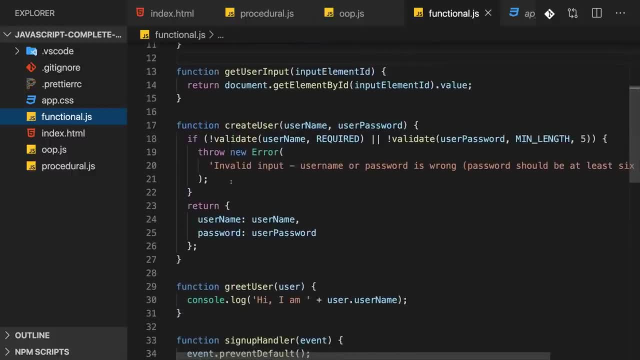 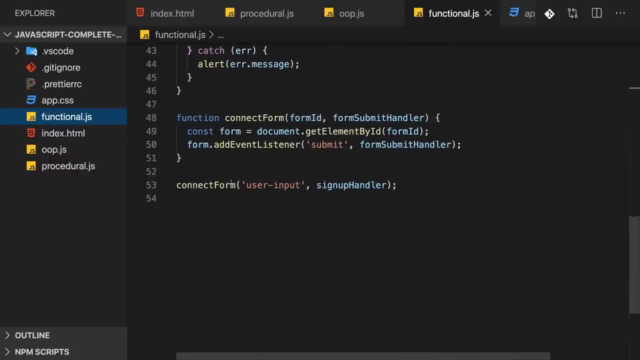 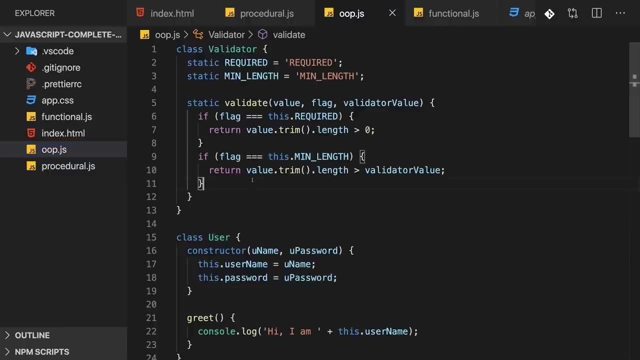 It's really nicely organized. It's very straightforward, Functions tend to be relatively small, if you're using this style correctly, And it also produces highly reusable code. Object-oriented programming was extremely popular a couple of years ago and it's still far from being not popular. 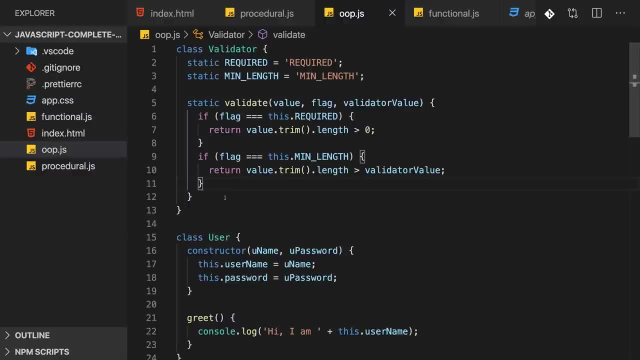 Don't get me wrong, And it does have advantages. It's also producing reusable code, and it splits your code into logical pieces. Now, with the classes, you sometimes have a little bit of overhead, which you don't really want, though. 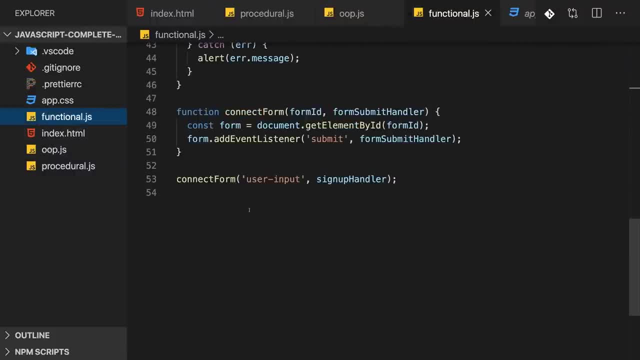 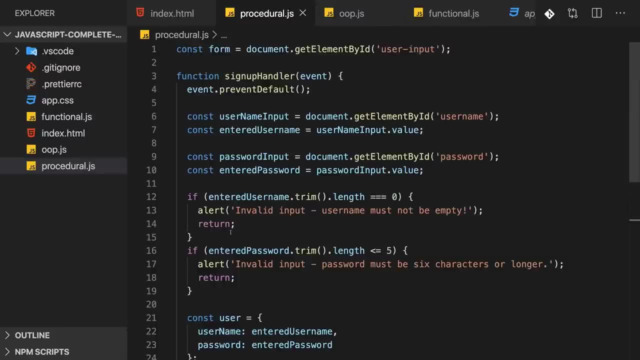 And sometimes it's easier to split it when following the functional style. The procedural style is not bad at all and great for some simpler scripts. The more complex your application gets, the more complex it might get to work with this style, though, Because you will naturally end up with 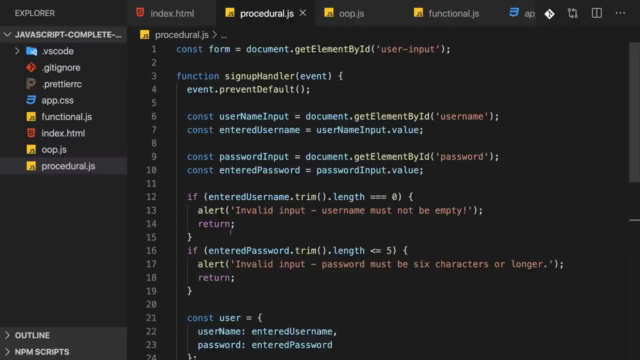 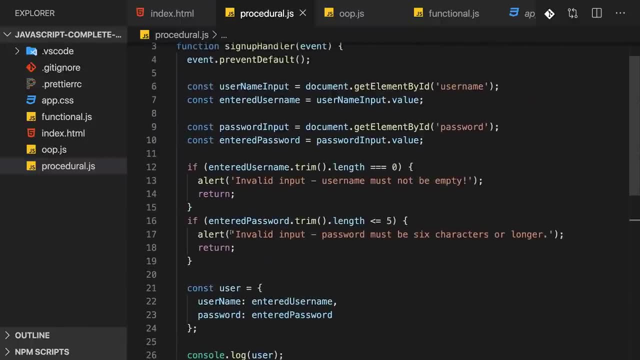 at least using some classes or some other functions to make it more readable at some point. Because if you only use this style and you write your steps, your code, step by step, your code can get harder to organize and to reason about. But again, here also, 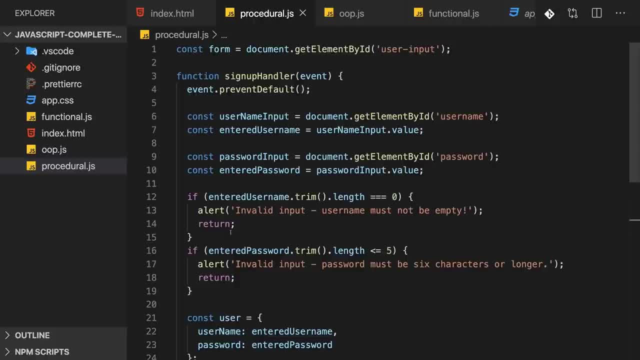 you can mix in more functions and so on and therefore also write great applications with the procedural style. I hope that this overview was helpful and that it helps you make decisions about which styles you want And, most importantly, that it helps you understand styles being used. 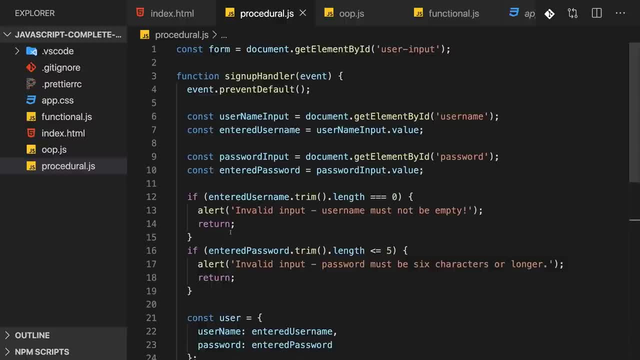 in different projects or in different frameworks you work with in your future As a JavaScript developer.